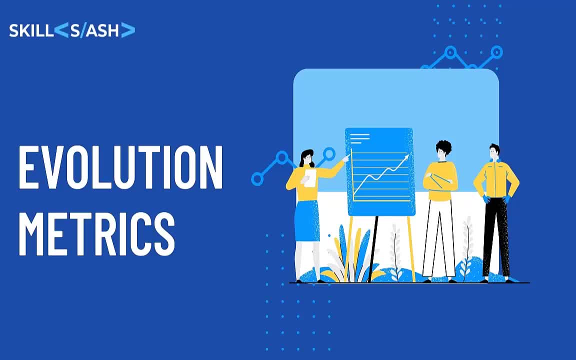 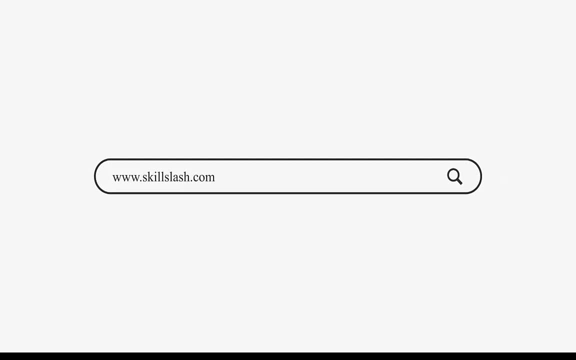 Evaluation metrics. This is the 12th. Now there are two important regression metrics, evaluation metrics for regression models that we look at The moment. you see it, you are going to recognize it. The first one is MSE, or mean squared error. 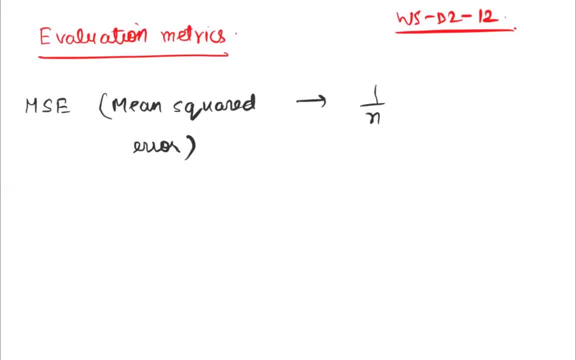 The formula for that goes like this: 1 by n, sigma yi minus yi hat whole square. This is MSE. Then you have RMSE, which is root mean squared error. It is simply under root of mean squared error. Then, as a competition, you have MAE mean. 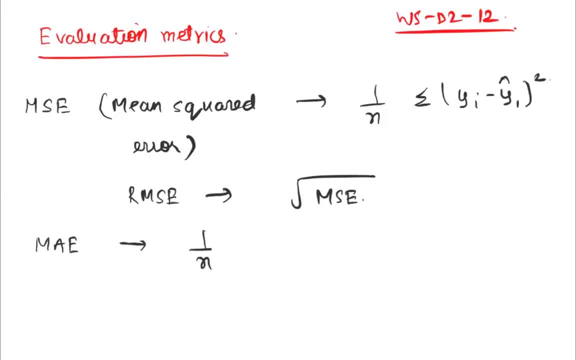 absolute error, which is 1 by n sigma mod of yi minus yi hat whole square- Sorry, not whole square Mod of this quantity. Everybody understands this by now, right? This is what You have done, this too many times now. This is actual, This is predicted, So for every. 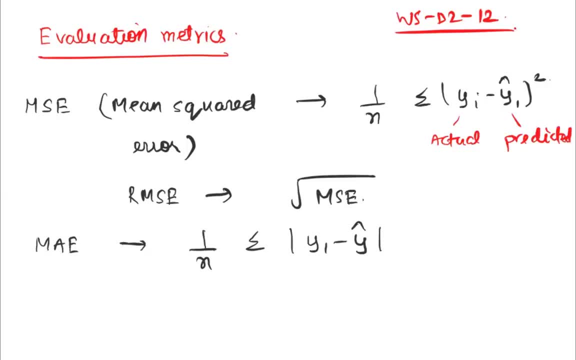 observation. you are computing actual minus predicted. Again, there can be some over predictions, There can be some under predictions. So you do not want to take a simple average of that number. You square that number and then take that average, or you take absolute value and 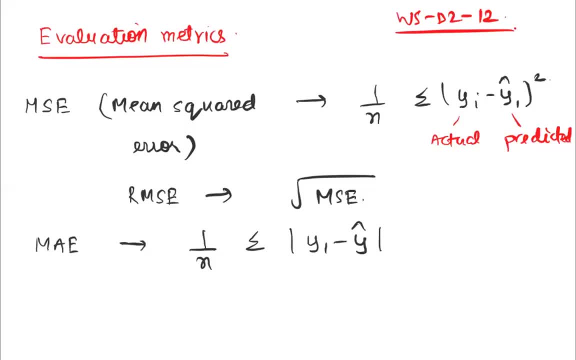 then take that average, So these come up as different terms. This is called a mean squared error. This is called a mean absolute error, MSE and MAE. MSE, again, is the squared quantity. It is like variance. You do not want to study this value in the squared scale, So you take 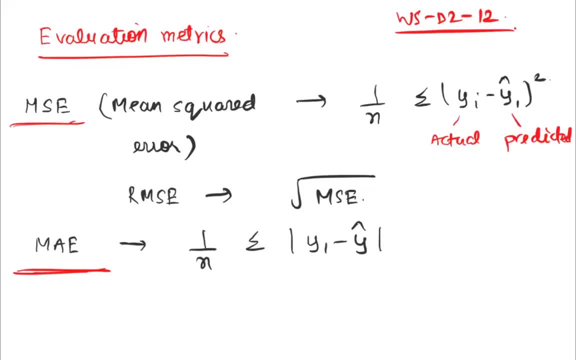 an under root of that and RMSE is present in the scale of the column that you are studying, So RMSE is the more used metric. But then the fundamental idea is same, as we discussed in variance when we talked about Gaussian and Laplacian ways of doing it, And that is. 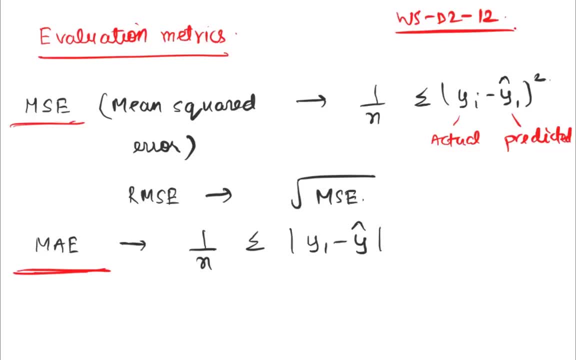 what exactly this is. This is absolutely clear, right? So this will we do after r square, or like: Yes, This is the final evaluation criteria for your model. You will look at the actual minus predicted. You'll take an average of that quantity, either after squaring it or 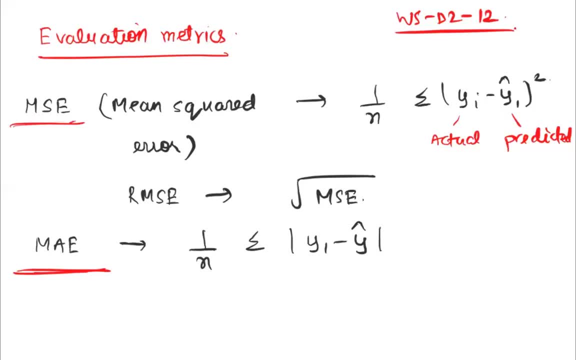 by taking up absolute value of it and you get a sense of the average error. Is there an acceptable levels defined? No, That depends on the. you know what scale of values the data has and everything You have to worry about. have to look at the context of the analysis and decide whether whatever error you are getting is. 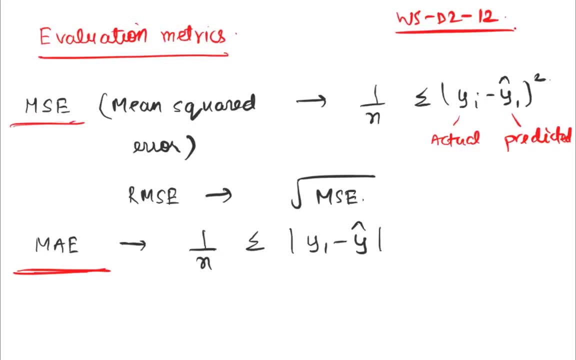 too much or too little. so let's say you are estimating sales and your average sales is, let's say, 10 000 units and your RMSE value comes out at 100. do you think this is acceptable? yeah, one percent is there. yes, your average sales is 10 000. so typically, any row, you has values in. 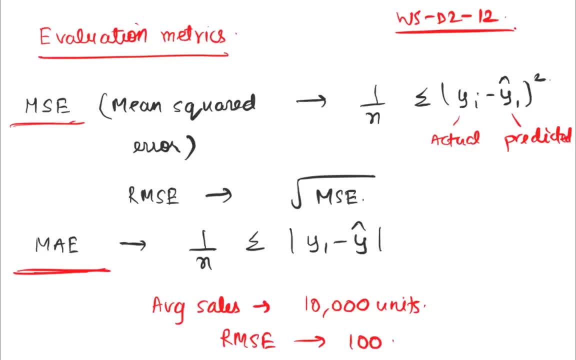 the range of 10 000 and you are getting an error in an average of 100, so that's one percent of not even one percent. no, that's little less than that. so you are getting an error in an average of 10 000 and you are getting an error in an average of 100, so that's one percent of not even. 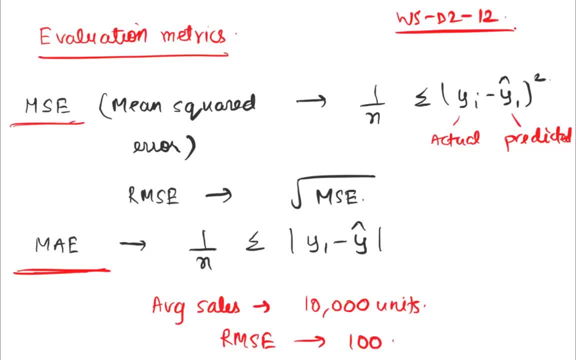 one percent, no, one percent. that's one percent of what can you know what you can expect. so that's good enough for you. so you, you look at your average value of the column that you are predicting, the value for, you get a sense of that column, and then you look at the RMSE. 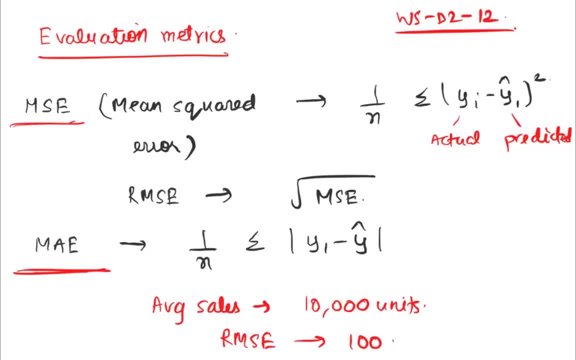 value. the RMSE value is by how you know, on average, how off you are when it comes to your predictions. if you were to predict 980, have you predicted 9080 or are you somewhere in that 980 region region? you're not way off from it. so the ideas you're trying to get out of this: 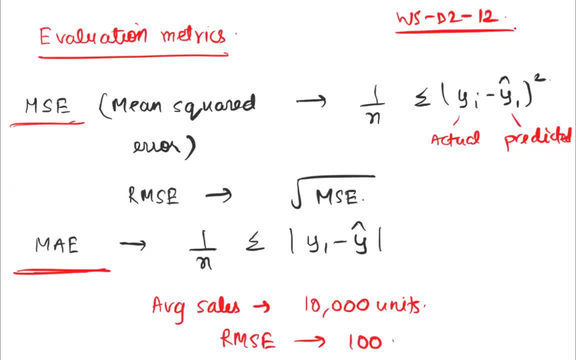 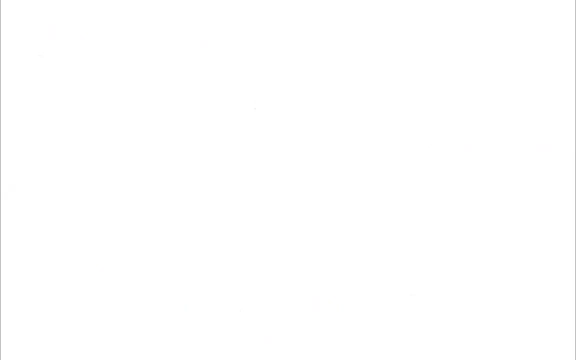 the fundamental difference between these two quantities is that MAPE or MAE, is slightly better when it comes to a few bad predictions in the model. if you have a few outlier values in your data, that's where you'll realize that MSE is better. so for that, let's look at an example. 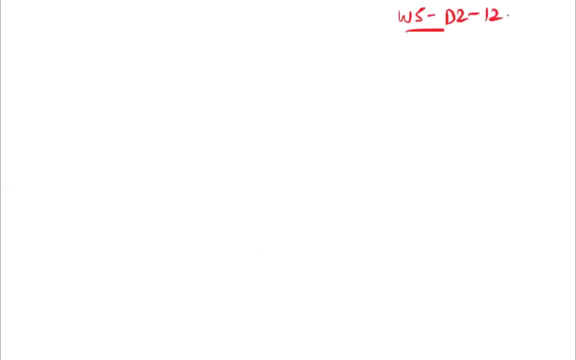 let's say this is your Y I and those values are 10, 20, 30, 40 and 50. then you have a Y hat. so this is a predicted value. the predicted values are 12, 21, 59, 43, 52. this is one predicted value. this is model. 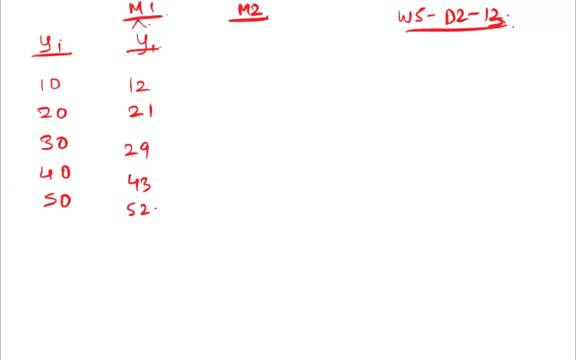 call it model one. then you have model two, which is also giving you your predicted values. those predicted values are like this: 20, 20, 31, 39 and 51. right now, which of these two models do you think is better by looking at it? model one, one, yeah, model model one is better, you say. 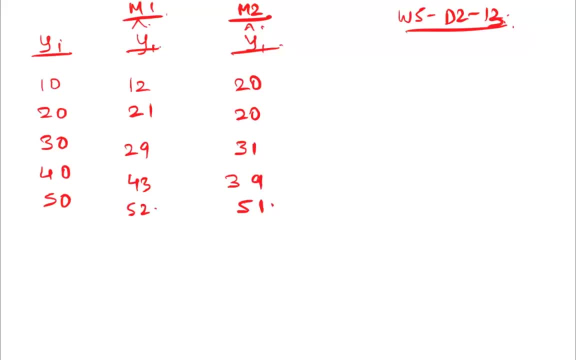 correct. yeah, now how poor is uh? we will try and check how poor is model uh two as compared to model one. if we think that model one is better, let's try and check that by looking at the rmse and mae for these two models. so what we'll do is i'm asking you to calculate the rmse value. 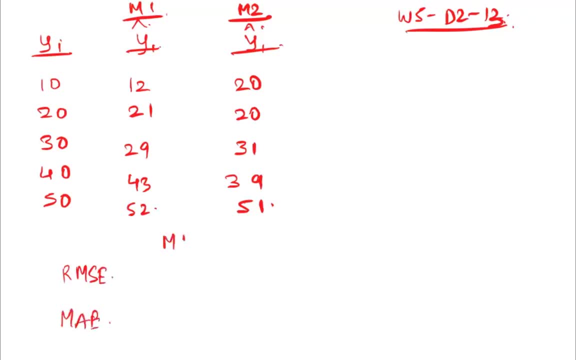 and the mae value for both these models m1 and m2. how will you calculate it? by calculating the errors, right. the first thing is to calculate the error actual minus predicted, minus 2 minus 1, 1, minus 3 minus 2. and here it's what minus 10, 0 minus 1, 1 minus 1. 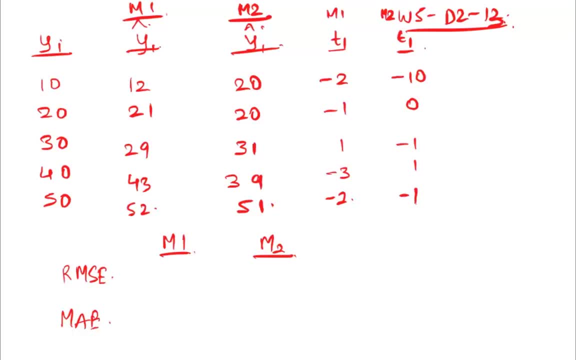 this is error of model 1. this is error of model 2.. now find out the rmse value and the mae value for both these models. first is 3.8. which one is 3.8? one, one by n, y, i minus y square. 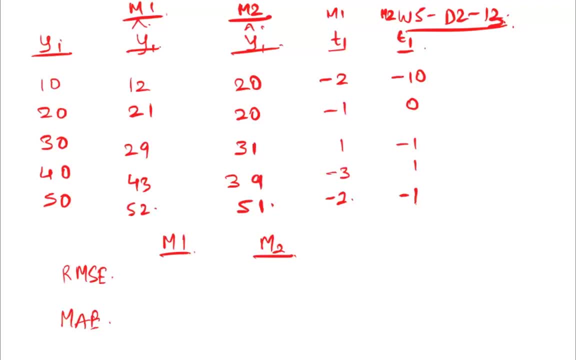 sigma of iron is nice, rmse of m1, no, no, rmse of m1 is 4.35, rmse of m1 is 4.35 rmse or mse rmse. so under root, you have done yes, yes, okay, let's see. this is the error. so square of error: four plus one, five, six, nine, six plus nine. 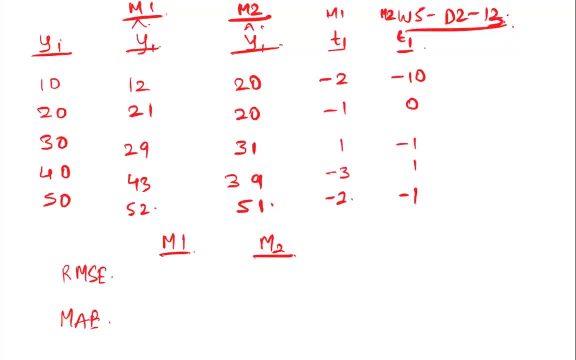 19 by six, four, nineteen, so it's nineteen by five, nineteen- oh, i'm now divided. so it's nineteen point nineteen by five is how much? three point eight. three point eight, three point eight under root will be how much? one point nine, five. one point nine. 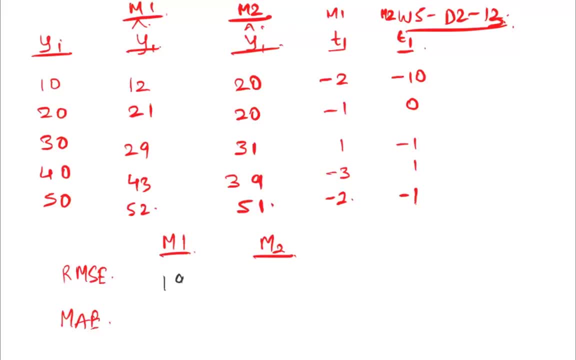 five. right rmse for this is one point nine five. what about rmse for this? this is hundred three, one zero, three by five. so twenty point six, four point one, four under root, four point one, four. yeah, now compute the mae. so this tells you what this tells you. 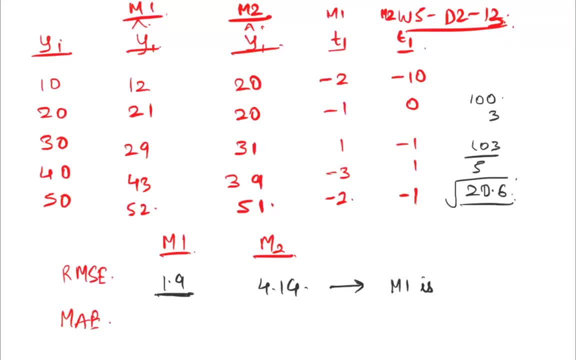 m1 is almost, is more than two times better. now let's look at mae mae, for these cases will be what? three, two, five, six, three, nine, nine by five is one point eight, one point eight, one point eight. yes, what about the model two? that's ten, three, thirteen, thirteen by five. all right, that's two point. 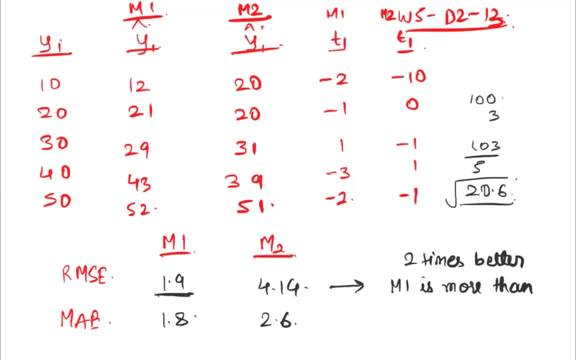 two point six correct. what difference do you observe here, or what is it that you can understand from this? now you've got an rmse and mae values? first of all, your assumption that m1 was better than m2. is that holding up? yeah, that's holding up. good, uh, what about? 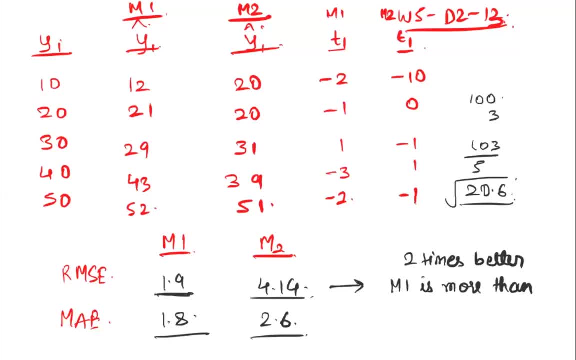 um, and there are two factors which are confirming that m1 is better whereas m2. there are two factors which, uh, in which you know we can say ma is better, but you know the, you know the opinion. for from what is it? the result of the accuracy test is very varied in m2 and then when m1 is there close to 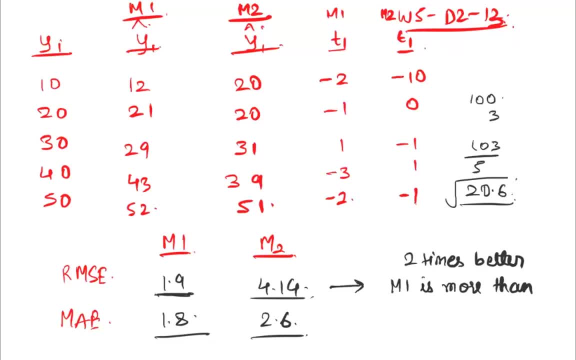 each to each other, rms enemy. so m1 is better. so when we have multiple factors, we can say that m1 is better than m2 is to confirm whether which model is better first of all. first of all, on both parameters, rmse and mae, m1 is better than m2. second, what you're realizing is that, as long as you know, you don't. 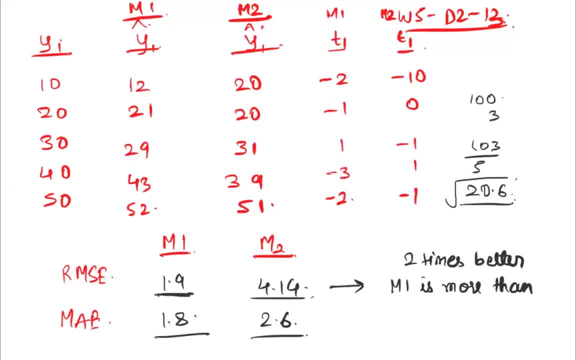 have any outlier values in your data, any outlier predictions or your antler values. uh, your model is doing. uh, your accuracy matrix? both the accuracy metrics are doing similarly. the moment that changes of them has an outlier value, your RMSE value suddenly shoots up right just because of one. 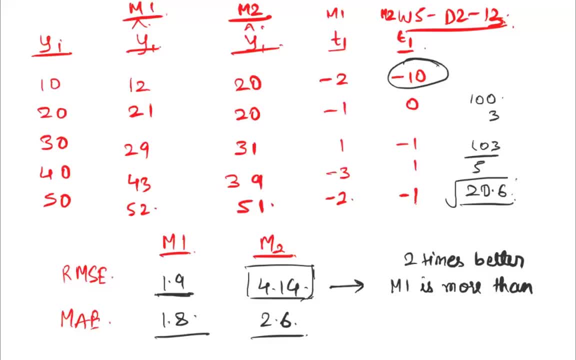 bad prediction. now, this model is not so bad. actually, just for one data point it's not done very well. for the other data points, it's actually done better than this model. this is better, this is equal, this is better and this is better. it's just that this is this. one is way, way better. 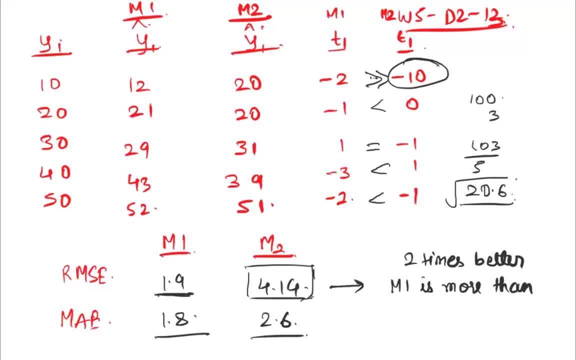 right. just because of that one value, your RMSE is suddenly getting inflated. because why is it happening? because there is a squaring happening in that process, because you're squaring the errors and then taking an under root that basically inflates that error, that one error is showing. 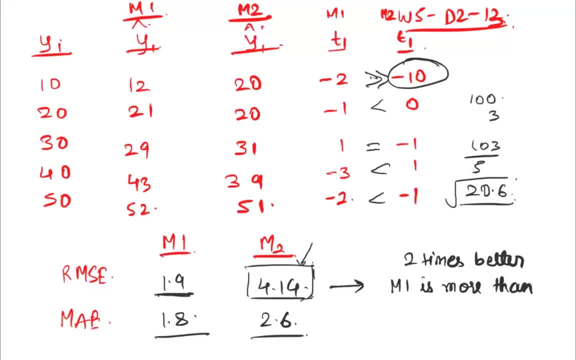 a heavy impact in M2 when you're calculating RMSE, but not so much when you're calculating MA. so MA is a little more resistant to you know, a few values becoming outliers and thereby you know the entire model results coming off as very bad. so instead of looking at RMSE in such cases, it's better to 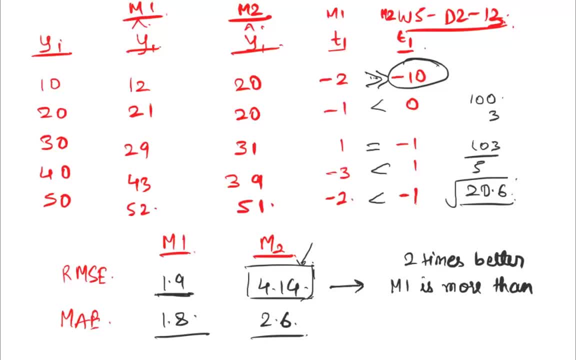 you know, gauge model results by looking at MAE 1.8 and 2.6. both of them are, you know, close enough measures. but 1.9 and 4.14 you can't really say that right with RMSE. you would have felt that. 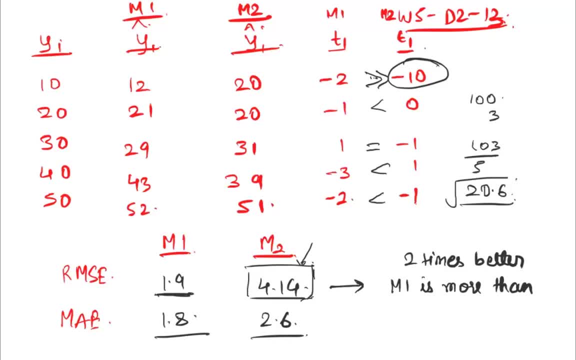 you know, M1 is very much better than M2. it isn't really. it's only better for one observation. actually, the problem is that for one of that one observation the other model is doing pretty poorly. does it mean that we should always prefer to use MAE over RMSE? not so much, but you will see that a lot. 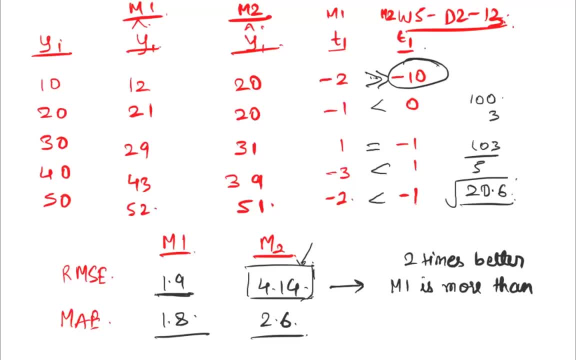 of ML, engineers prefer MAE over RMSE. statisticians always used to prefer RMSE or RMSE. now you will see. machine learning practitioners are more in favor of MAE, but they can't. there isn't any solid argument in either one's way. obviously MAE, because it's not squaring and taking under root. it removes. 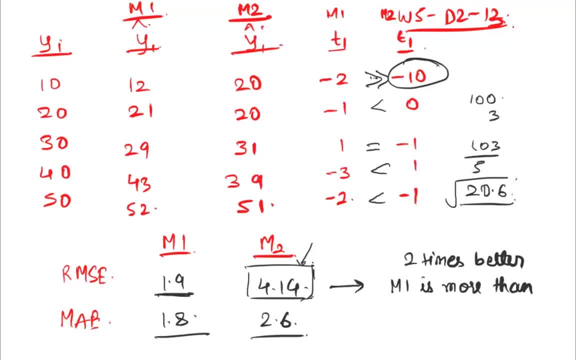 an unnecessary step that can magnitude the that, sorry, that can magnify the magnitude of the error. so it's an unnecessary magnification of error. so smart thinking tells me that MAE is more preferable. right, you can make your choice for yourself. everybody can have their own arguments, but you know, for me I like MAE more than I like. 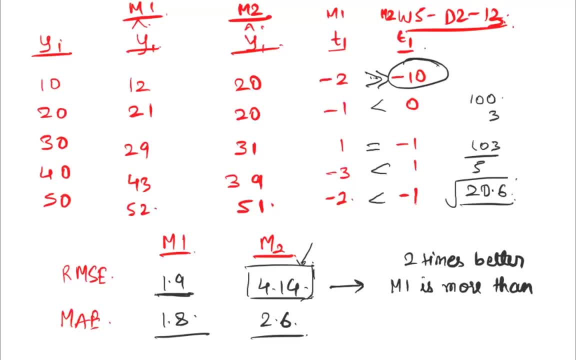 RMSE. so, Rahul, just like in R2, it was like explaining the variability of the independent variable. so here it is better than M1, is better than M2 two times in terms of like. the error is half of almost less than half of M2. RMSE is the average error that it is making right, so we can say the independent. 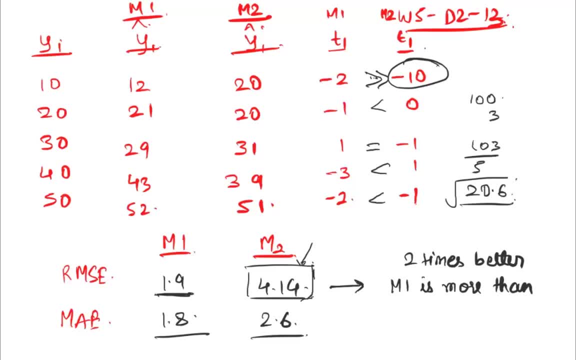 Y column is the model two on an average is off by four units, and model one on an average is off by 1.5- 1.9 units. when it comes to predictions, the actual value by which it's off is minus is two units, one unit, one unit, three units and one unit. 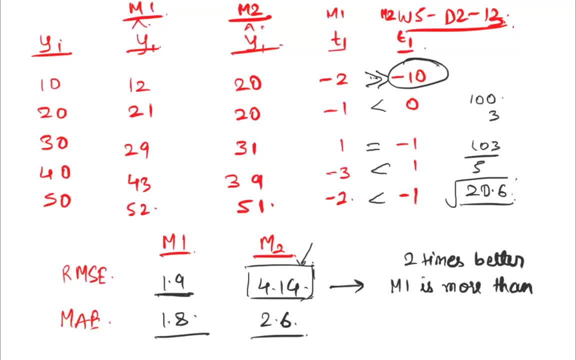 we are computing an average of that in two ways. one way we are squaring and taking an average in, then taking under root. in another way we are basically taking an absolute value and taking that- so one units like average- off by four units of the dependent variable. 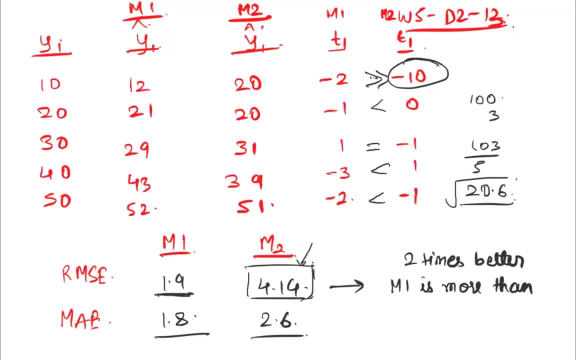 correct, correct dependent variable. when you're making a prediction, you're typically off by four units. okay, good, that's what it means. take any question about this. uh, Rahul, but this still leaves it at large, you know, to decide which method to choose between RMSE and ME. 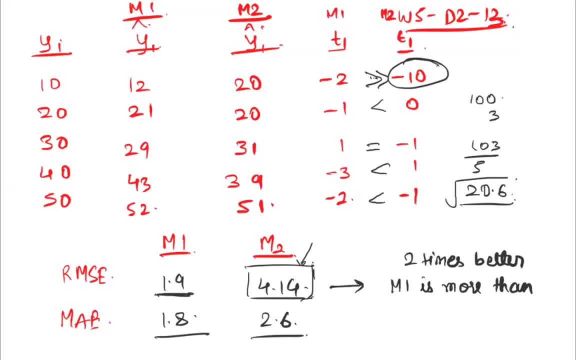 no, no, can you come again? I couldn't understand it. so this still leaves us, at last, you know, to know decide whether which one is better. I mean, you know, based on what the statistician says, or what business is comfortable with. I don't have much of a say, but you can make your arguments for both. 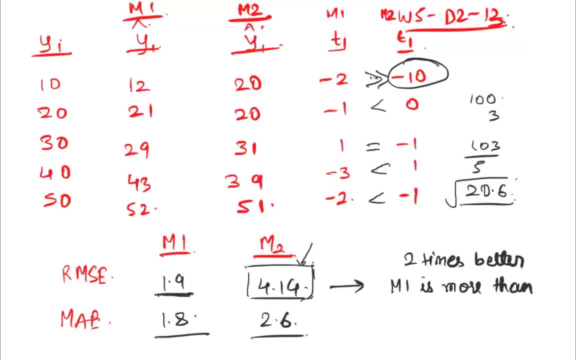 the cases I like a more than I like MSC, just because I feel the squaring is an unnecessary step, correct, okay, magnification of error. so I feel MA is just as good a uh, uh, uh. representative of model accuracy, if not better. if you feel you have, you are more in favor of RMSC. 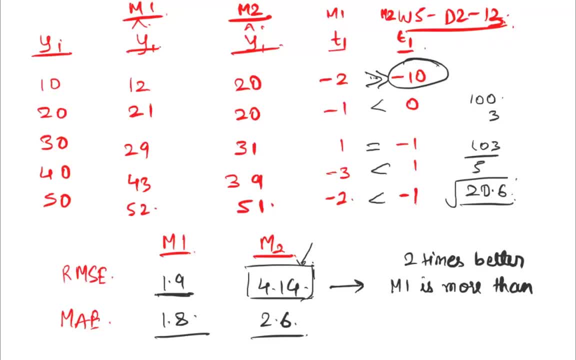 you have to present an argument in that favor. I think ma scores over RMSC, but both of them there's not much difference. these are very good comparative metrics when you're comparing models. directionality of impact will never change. it's not like RMSE will tell you. 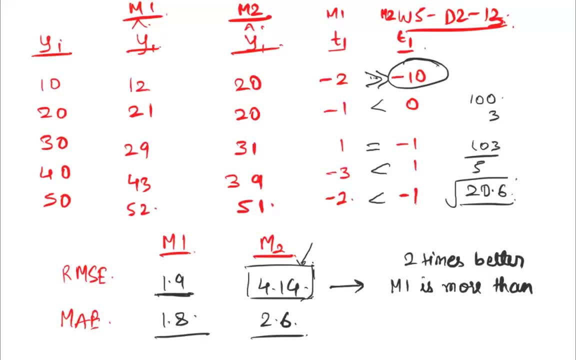 that m2 is better and ma will tell you m1 is better. that will not happen. so, as far as directionality is concerned, when you're comparing models, it's more or less okay. yeah, what you're worried about is what you finally need to present to the business. so what's going to happen? you're going to have a 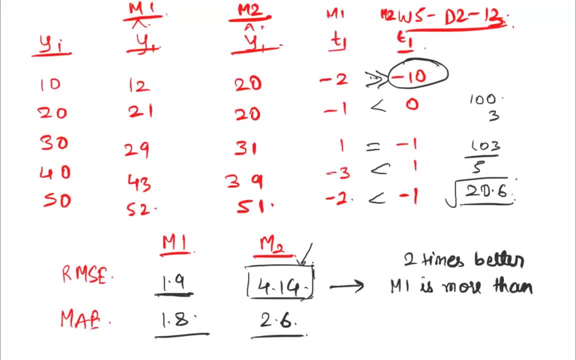 fly with the business. yeah, but as I said earlier, can I use both RMSC and MSC to make sure that you know? yeah, I mean both are saying the same thing, which means that even after squaring- why not, why not? that's the same way. yeah, why not? yeah, that's it for me. thanks, okay. 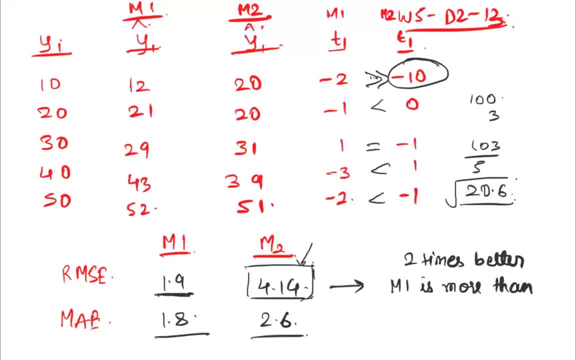 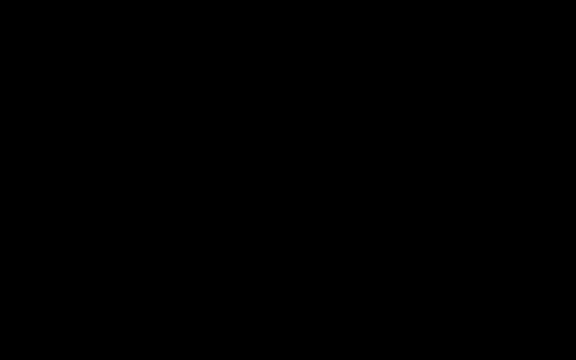 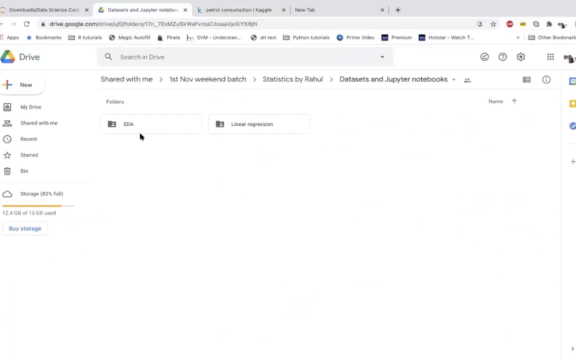 all right then. so we've completed this discussion. for now, let's go for a break. let's come back at 2: 30 and we have a the folder. inside that folder there is Jupyter notebooks and data sets. that's one: datasets and Jupyter notebooks. you had one for EDA, now you have one for linear regression. 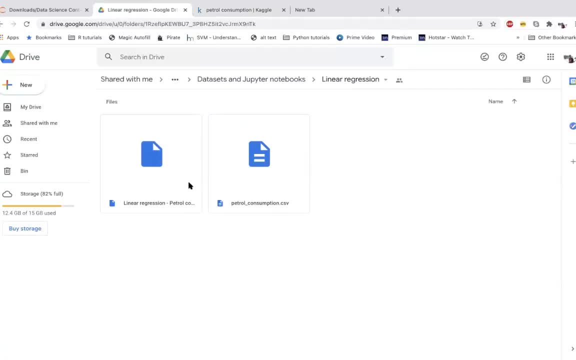 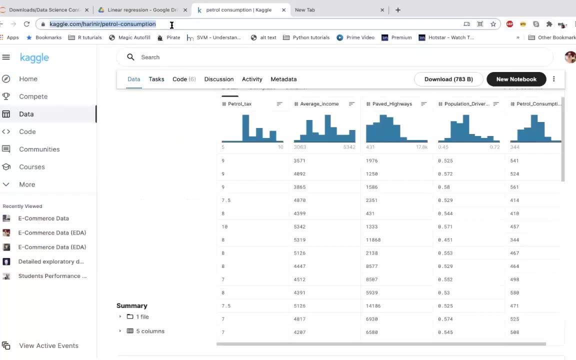 go to that folder and download both these files. one of them is the python file and the other one is a csv, which is the data set itself. I am going to share the Kaggle link for the data set. you can download it from here. but you know it's best if you get it from your drive. that'll be. 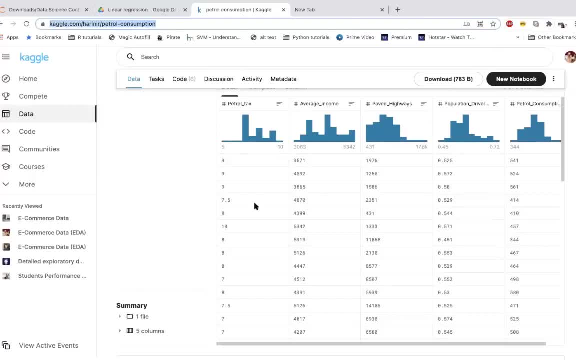 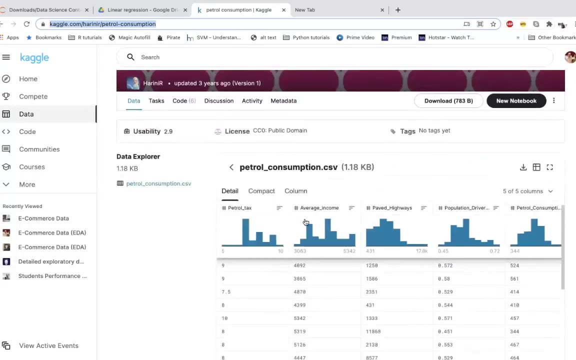 easiest. okay, so I passed the Kaggle link on your chat so you can get from there also. so get your data set. the data set is a simple one: the only five columns inside the data set is, one of which we will use as the dependent variable and the other four we'll use as. 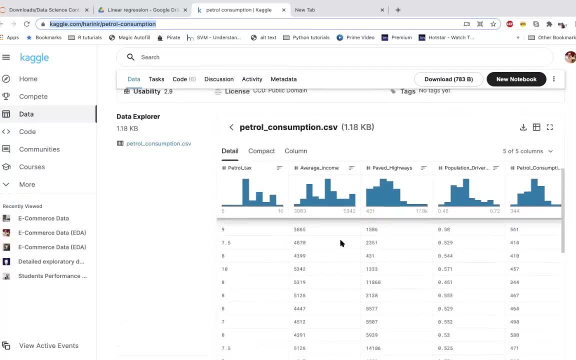 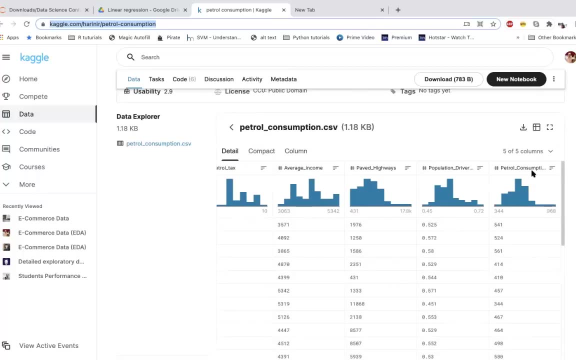 independent attributes. so our dependent column in this case is the petrol consumption column, which is so. we've got data for 48 states in the united states and we've got petrol consumption levels in gallons. we've got population driver license, that's the percentage of the population that has a driving license. 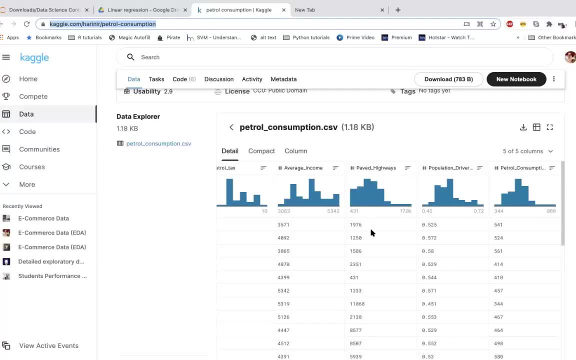 in that state. then you've got a number of paved highways that you've got in the state. you've got the average income of the state and the petrol tax that is imposed in that state. so you've got four independent descriptive variables: petrol tax, average income of. 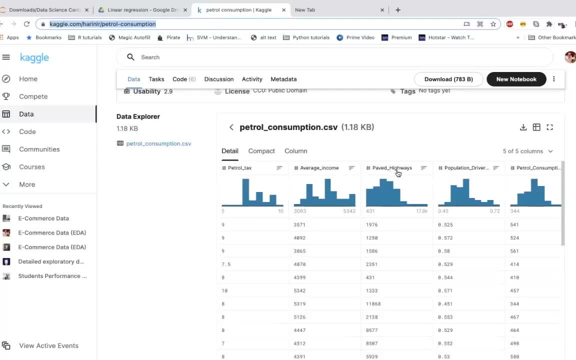 individuals in a particular state, paved highways, the number of paved high days in highways in a given state and the percentage of the population which has a or holds a driving license. based on these four factors, you've got to pay for the driving license. based on these four factors, you've. 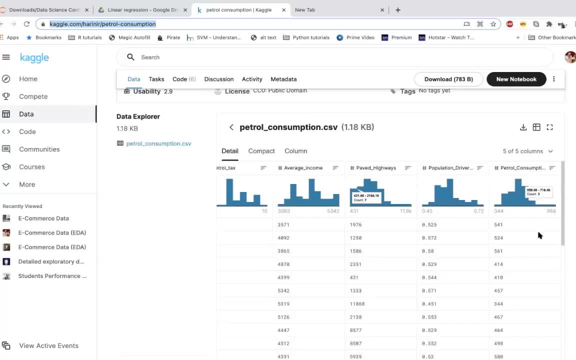 got to pay for the driving license based on these four factors. you've got to pay for the driving license paid for on the stretch. so at this stage the consumer candidates need to predict the petrol consumption level of any given state. that's the objective of this case. we're trying to 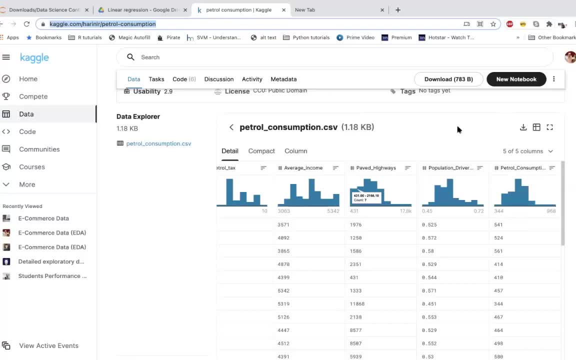 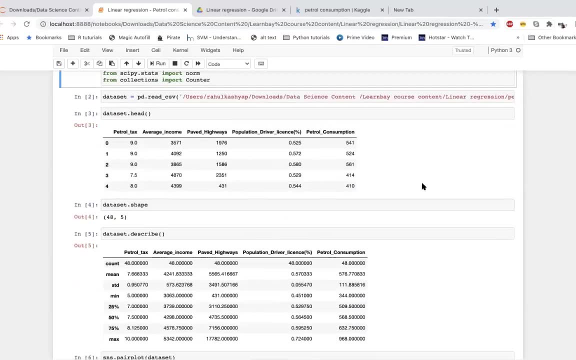 build a simple- uh- linear regression model, not a simple, but a multiple. you start off with simple, we go over to multiple linear regression model, so we'll build a multiple linear regression model to try and do this, okay, so i think you looked at describe and then you go on. i think the person who was talking about this be happy to do it. i think this, this camera was working like a Harlem model. hey, since the card is moving, this is how you can predict it. so it will predict the Kevin Martin model right now. if the law falls that it will make myself have with it. 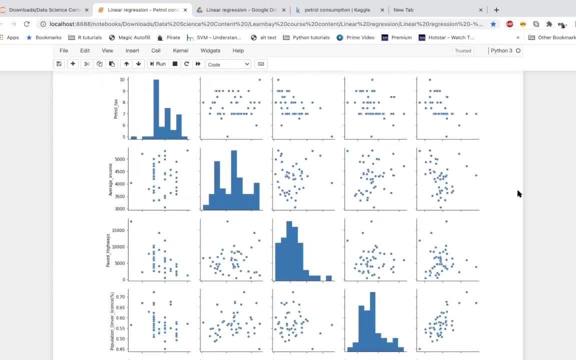 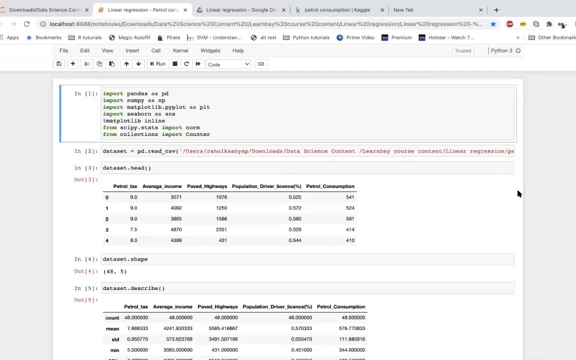 people would have looked at, described, tried to do as much understanding of the data set, but then what? what are the next ideas that you would look at? what are the next things that you would want to do in the context of this objective? correlation, yeah, correlation between the variables. try to 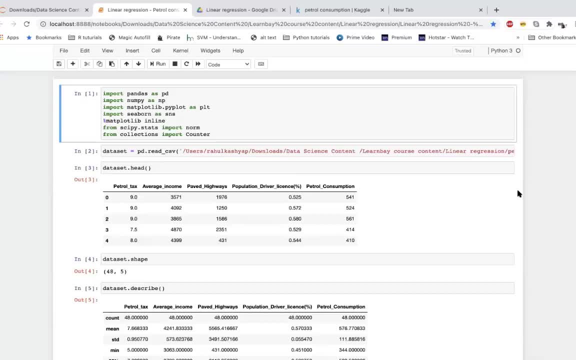 understand at a high level. what do they and how do they influence each other or not correct? so you now are interested in trying to understand whether these variables are related to your y column or not. so my petrol consumption is what i'm interested in. i'm trying to understand if 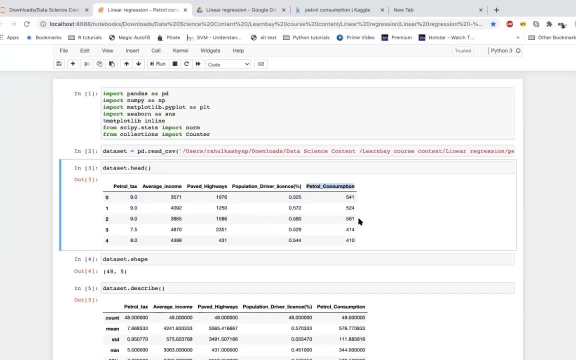 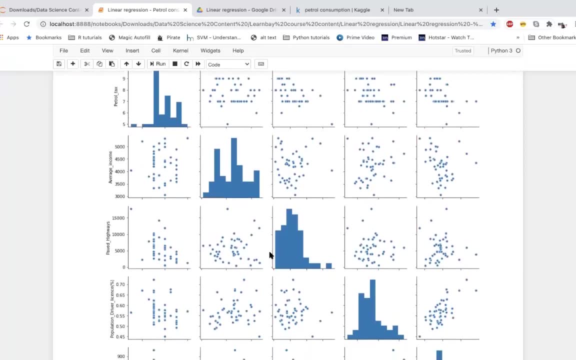 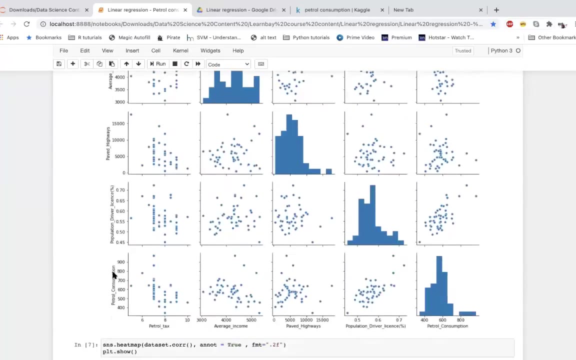 these columns have a significant correlation with petrol consumption, which can be- uh, you can start off that with a pair plot. a pair plot basically gives you a scatter plot. it gives you a scatter plot of all combinations. you have petrol tax, average income, paved highways, percentage, driving license and petrol consumption, in the same order here and on this diagonal, whatever combination. 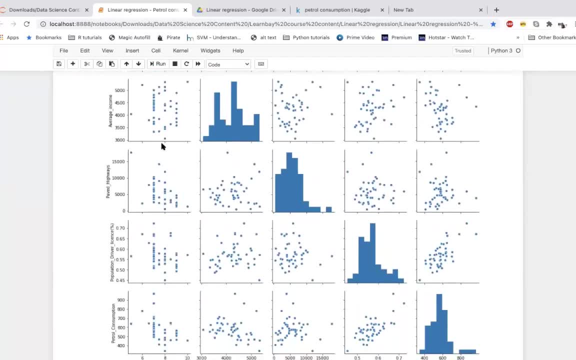 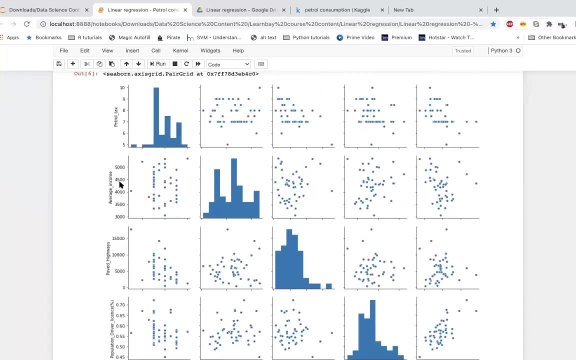 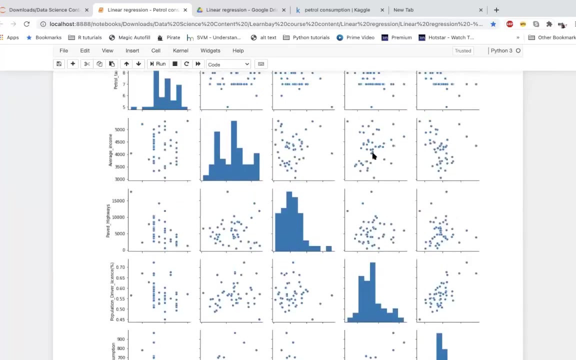 you have. you're looking at the scatter plot for that particular series. you will. you can look at scatter plots that might be helpful in trying to identify relationships. so this combination- we are looking at average income and population, driver license- what do you think the correlation in this would be a linear 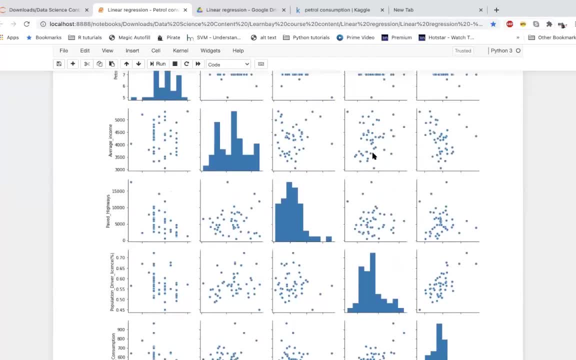 average income and population's driver license. it's it's it's mixed, i mean it's a little tricky to identify. it seems to be almost like you know. it's in the same scale throughout. almost there isn't any distinct pattern that i can find here. as compared to that, if i look 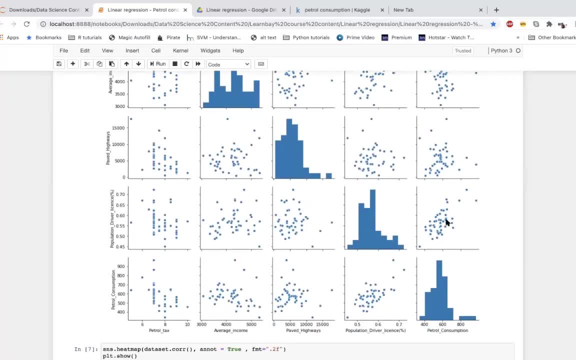 at this one. yeah, look at this scatter: population's driver license versus petrol consumption. what do you think about this scatter? they are linear, like highly correlated. it seems positive, direct, positive relationship- yeah, there seems to be some. you know, i can see a line being fit on this uh pattern. right, i can see that the line easily gets fit here. 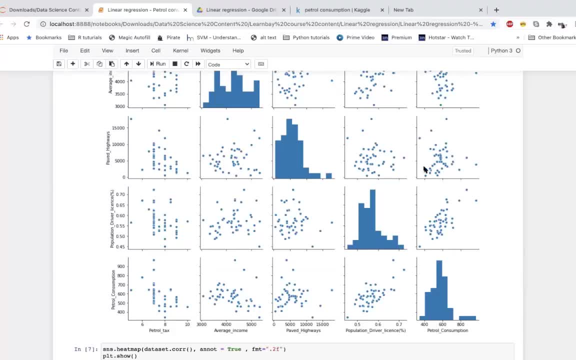 let's look at other combinations with petrol consumption. what do you think about paved highways? does this seem to have an impact slightly? yeah, i mean it's a little sorry, it's a little very. there's no distinct pattern as well. it seems a little positive, though it seems like you know as i go. 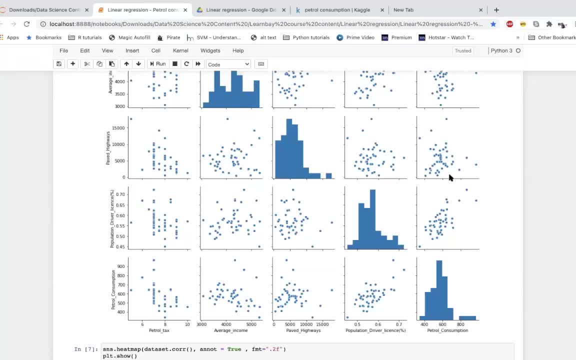 further away on the x-axis my lower values have sort of disappeared right. this range has become a little empty. whatever values i see are a little higher on the y-axis as i go further down the y-axis and then i go further away on the x, so it might seem like there is a little bit of a positive. 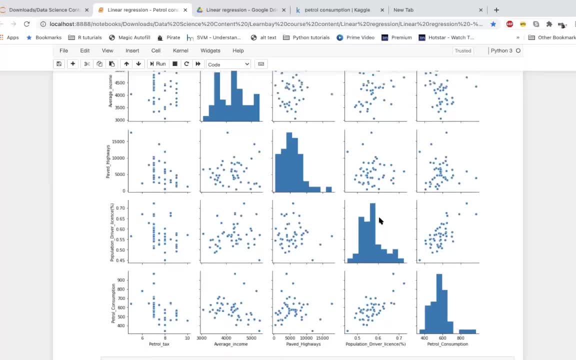 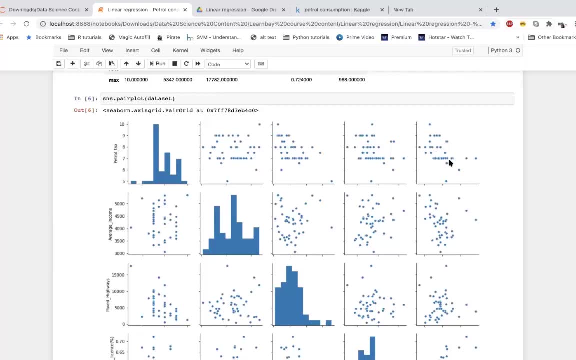 trend. but you know hard to say, you can't really comment very confidently here. you've got petrol tax. so it seems like at the lowest petrol tax you got the maximum consumption. that's quite, you know, makes sense. what little lesser as your petrol tax goes up. so as your petrol tax is going up, you've got a lesser. 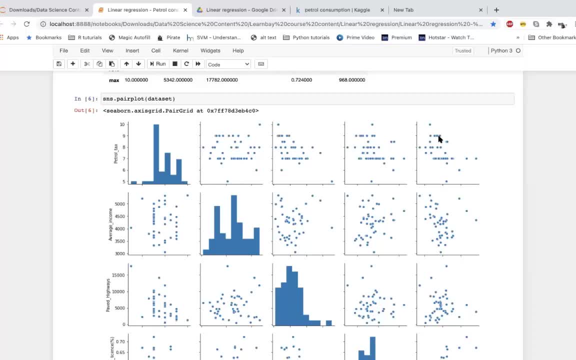 density and the lower value for petrol consumption. that also makes sense. so there seems to be a negative sort of correlation. right, if i were to expect a correlation, i would expect a negative correlation, would it? would i? yes, yes, and the tax rates will influence the. what is the last? 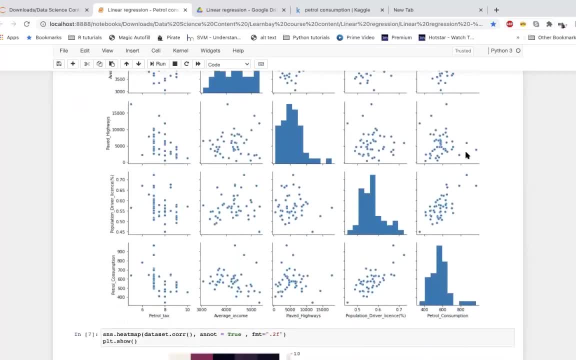 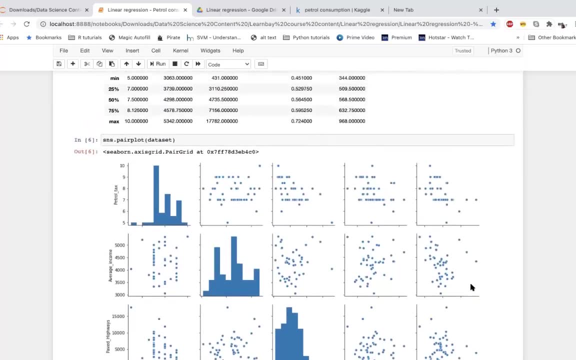 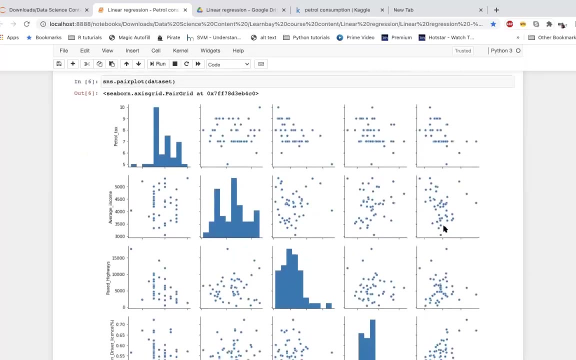 column. so if you can go and scroll down please, that's the consumption, that's the way, yeah, yeah, yeah, higher the taxes, lower the petrol consumption, correct, correct, correct. higher the petrol tax, lower the petrol consumption. so i'm expecting a negative correlation. sorry, a very basic doubt. 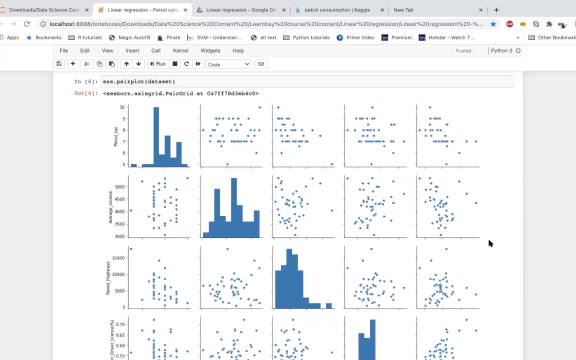 petrol tax is a discrete uh variable. that's why we have like lines like: actually correct petrol tax cannot take values. in this, between this, this middle area, you cannot take value. so you'll never get a dot here, because scatter plot is simply x comma y, so the x value will always. 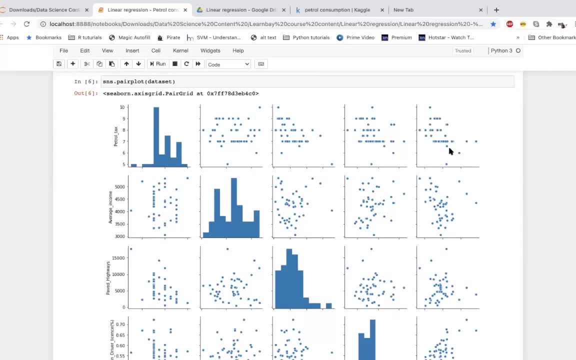 y value will always be on these scales. so you've got lines like that, but the density on those lines will suggest how many values are present at that point and you know their relative position. x axis will indicate how much are they using. who are there? so there are some people here who are using. 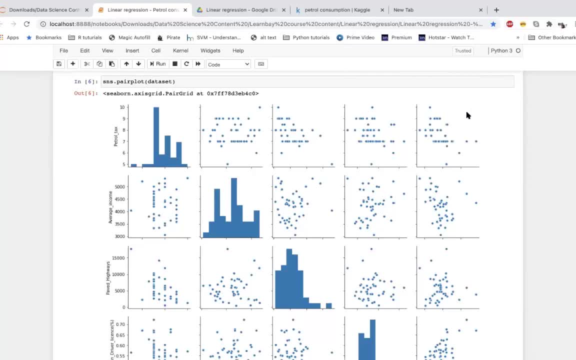 quite high amounts because they've got lower taxes. you don't see these high amounts in the upper region here, which means that your petrol tax at when you got higher levels of petrol tax, you don't see too many people. uh, you know purchasing too much, you know having too much consumption on the x-axis here. 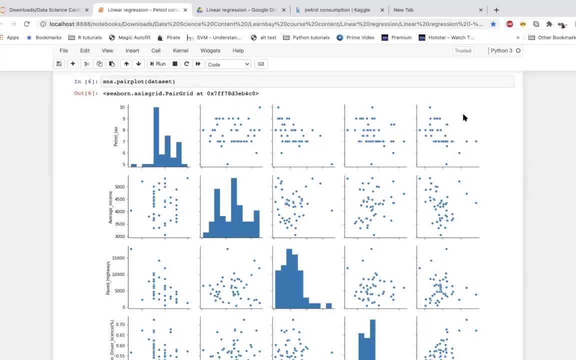 so that is an indicator that you know sort of it's a negative trend, more or less. yeah, so we can actually use a pair plot for discrete variable as well? i just yeah. i mean it's a little difficult in the initial stages now, i've been looking at these plots for a long time now, so 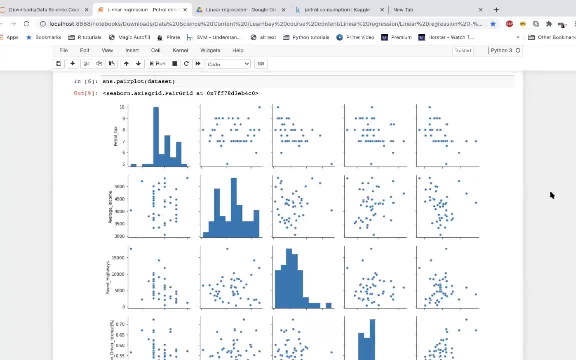 for me it's a little easier. maybe at this point for you also will get easier. maybe in three months or six months. the more you look at these, reaction also will get easier, maybe in three months or six months. the more you look at these plots, the more you will be able to read out of them. but your apprehension is correct in thinking that you know. 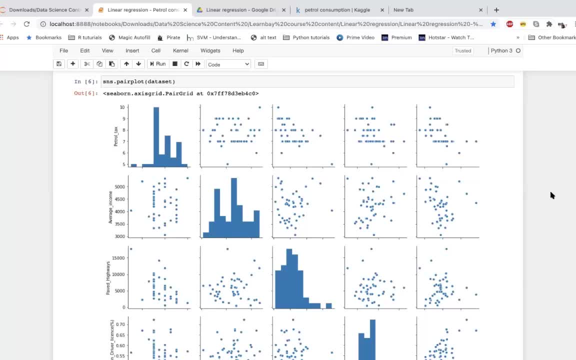 if you've got a discrete variable and a continuous variable, these kinds of scatter plots and correlation numbers, these aren't very strong indicators of what the real relationship is, because one of the variables isn't behaving in the way that it is supposed to be here, correct, yeah, yeah. 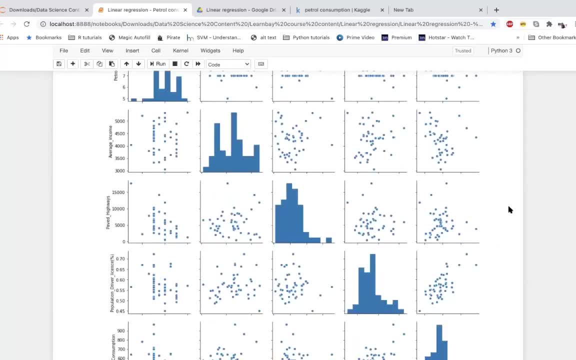 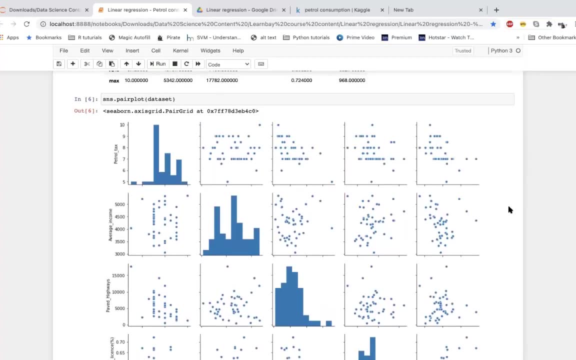 okay, just a question. So scatter plot is not. it's different from the dot plot, right? The very basic thing which you put in X and Y, Scatter plot is no. this is: these are scatter plots that are being drawn, So we are doing a pair plot. 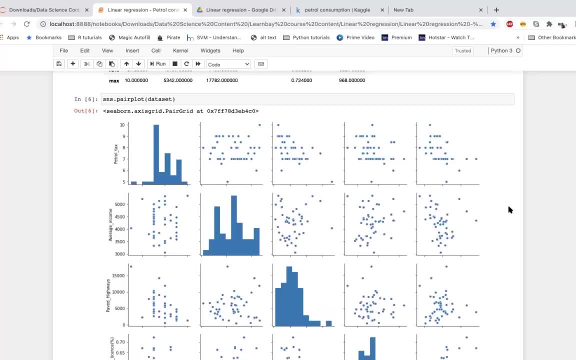 Pair plot basically does works on a data frame And for all combinations it gives you a scatter plot in the middle along the diagonal, because it knows that you know petrol tax and petrol tax doing a scatter plot will do what? Okay, histogram yeah. 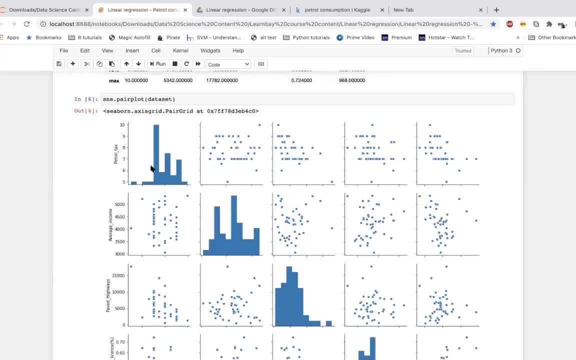 So it's better to just do a histogram. A histogram is a better- you know- alternative to drawing. you know X, comma, X graph, And I should know this. sorry if I missed this earlier. The scatter plot is nothing but X and Y plot. right. 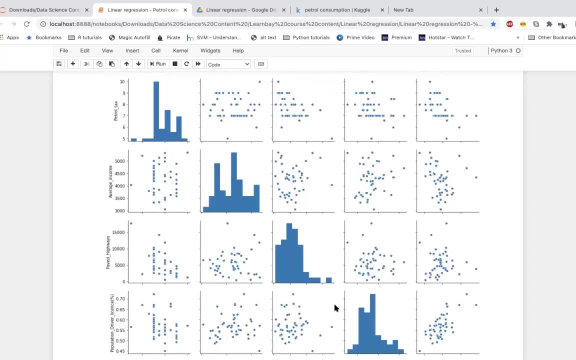 For each and every data: Correct, correct, Simple X, Y. yeah, yeah, Simple X, Y, Cartesian coordinates. you're simply representing those points, That's all Okay. Okay, so for every variable. we've sort of understood the relationship with petrol consumption. 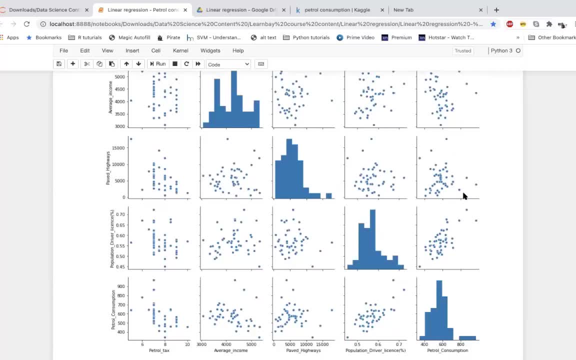 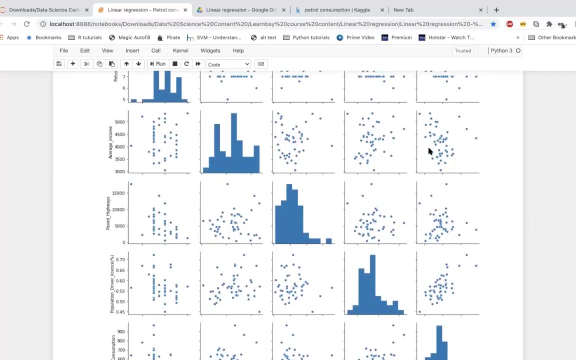 Looking at the scatter plot. Just by looking at scatter plot, we have a fair sense of what it should be like. We'll now try, and you know further. you know, use our learning. So about average income, we've not done that. 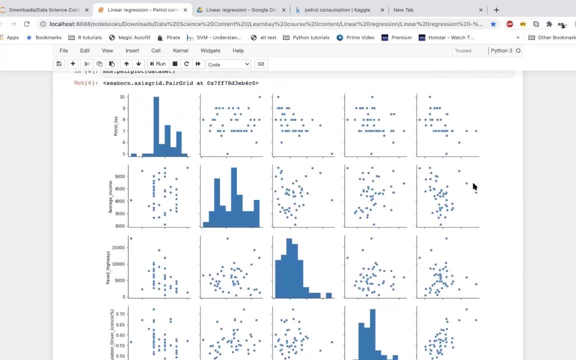 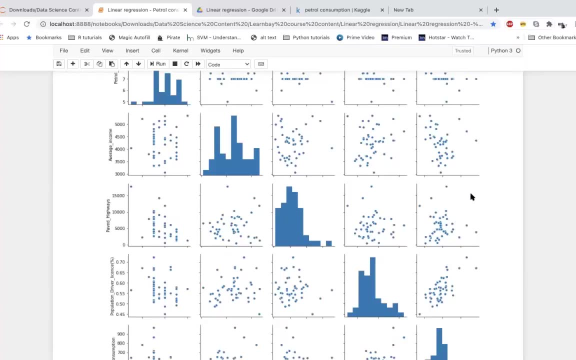 We've said that for petrol tax it should be a negative sort of relationship. Paved highways, you know. it seems like it's a positive sort of relationship. Not so much. no, Yeah, Maybe not positive Or close to positive. 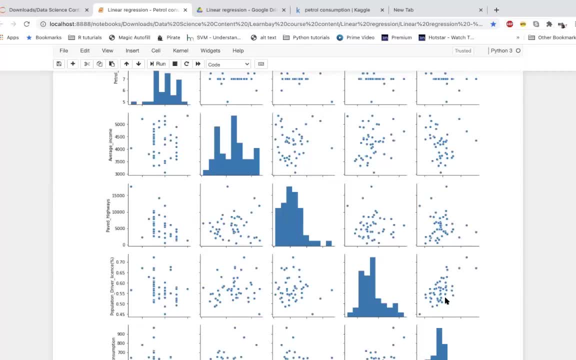 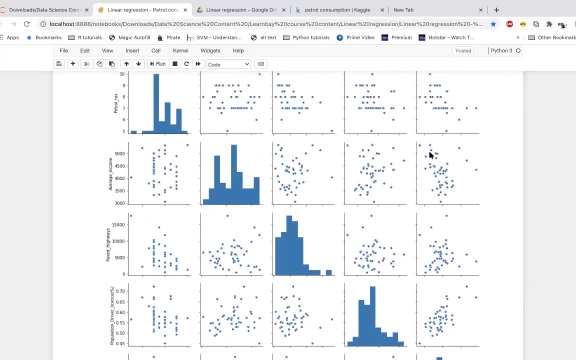 Close to positive- A little positive, I would say. For this. I can clearly see a positive trend, Something that is identifiable, Just for average income. we've not made a hypothesis For average income. what would you say from this scatter plot? 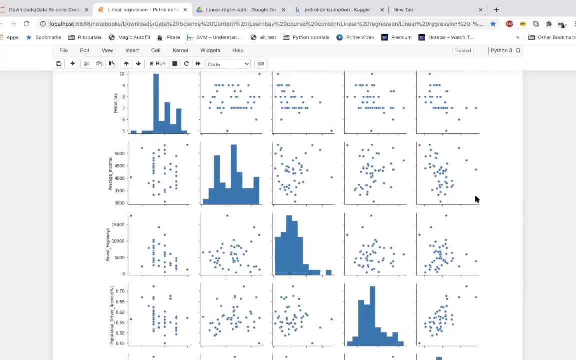 What do you think Doesn't- doesn't- I mean average income, doesn't influence. The only thing that I can say is: in this region, there's nothing that I can read out of this region. This region seems completely hopeless, But then these three points give me a ray of hope. 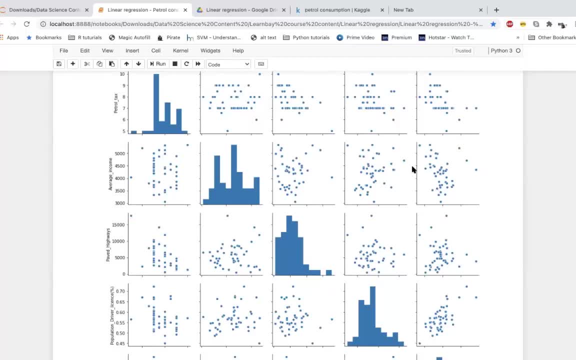 They tell me that at high values of X The values of Y are also very high. But such high values of X do not exist at low values of Y. So I can think of maybe a little bit of a positive trend maybe, And then common sense tells me: okay, more average income in the state, more petrol consumption. 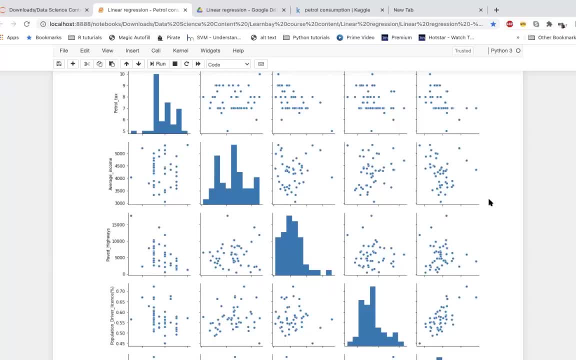 Makes sense. But if you see the clustering, like you know, if you were to draw some lines of the maximum fit, like for the entire thing, won't you think that this is negative? Say, for example: Yeah, exactly. 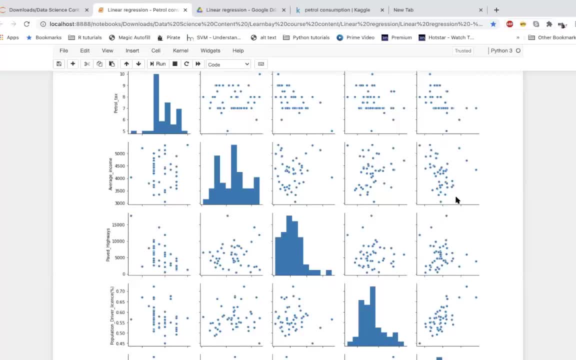 How you drew that? Yes, Something like this, Yes, So won't you say that it's negative? Makes sense also because the people with more income will be within the city limits and the drive distance. what he does will be pretty less. 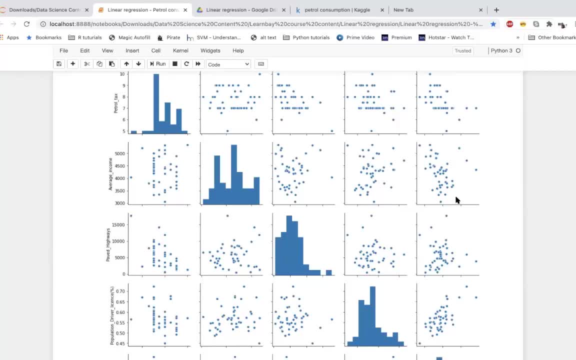 Right, I can't disagree with that. Looking at this curve, I'll have to agree that yours might be a stronger argument than mine. You know, the one that I am saying with these three points seems to be. I would probably go with your argument saying: average income and petrol consumption sort of show me a negative trend, which is unlikely, but it is what it is. I was kind of trying to justify that answer, because if you have, like you know, higher income, you tend to be more towards the city and your driving distance. It's a far-fetched idea, but the difference is a difference. 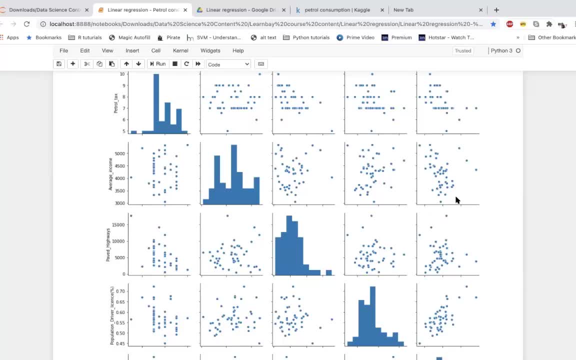 Yes, yes, that's a good defense, actually Good defense, yeah, All right, So I think. so we've sort of gotten a conclusion. We can also sort of understand and try and learn about relationships between independent variables. But you know, we don't want to spend that much time because we've got a mathematical tool to do this for us. 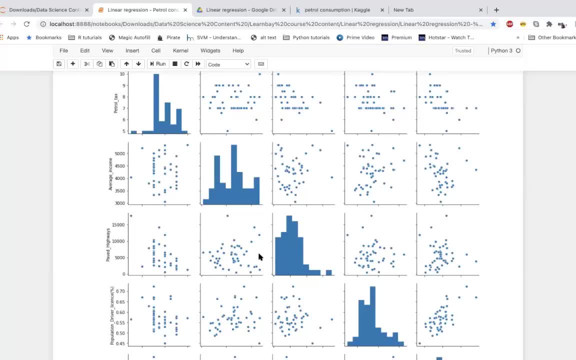 We were just trying sort of doing something that could help us do a double check with that tool. We already have correlation right So we can look at correlation numbers and sort of get a sense of any linear relationships which exist between any combinations. 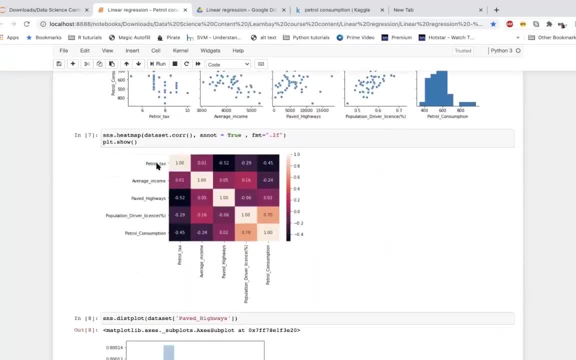 And that is what we're going to do next, which is a correlation plot that again draws the same matrix And at these points, it tells you the correlation between any two combinations of variables. Good, This is much better, much easier to read. 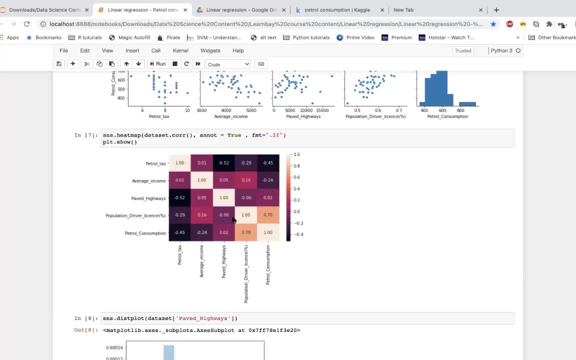 From here. if we find any relationships in independent variables, we can go and look at that scatter plot and sort of verify it again. But this is where we start our analysis from Now. looking at this histogram, What seems to be happening? 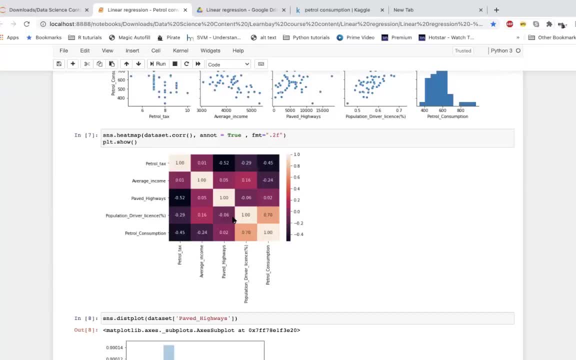 Petrol tax. you're seeing a strong negative correlation, right? I would say strong Minus 0.45.. So our intuition was correct in the scatter plot. Yes, Yeah, Our intuition was correct in the scatter plot in thinking that as the petrol tax increases, your petrol consumption decreases, which is evident in a strong negative trend. 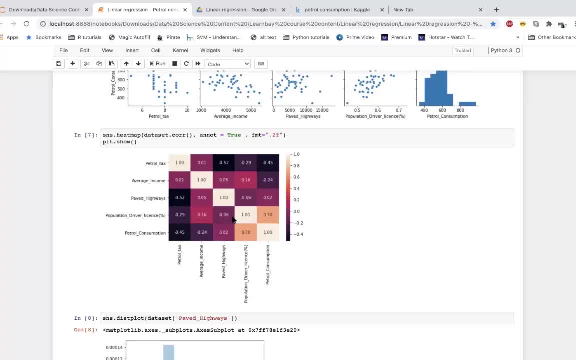 Average income again is a negative trend. So you were indeed right And it's the negative trend which is more prominent Here as compared to what I was saying, and that's clear from these correlation numbers. So the correlation number is saying that as your average income is increasing, you have negative trends in your negative trends in your petrol consumption. 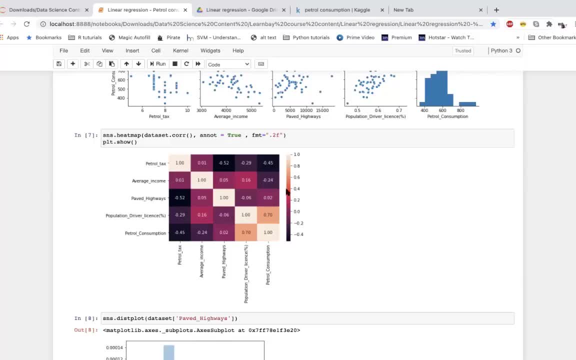 What about paved highways? Okay, Paved highways has a small positive sort of value. Makes sense. if you've got good highways, You know People might love driving and just for that you know so many people are driving and that might increase petrol consumption. the more number of highways- good highways- you've got. 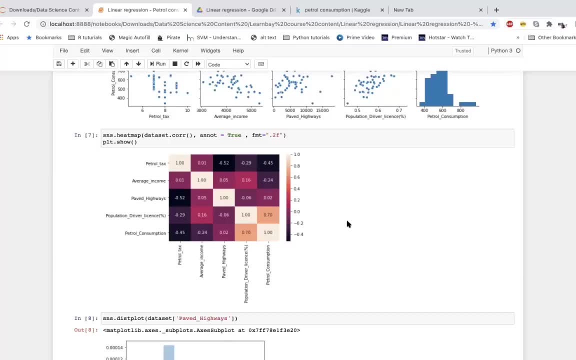 So there might be reasons to justify it. The simple fact of the matter is you don't really need to justify it because the number, the magnitude itself, is so low that you know it doesn't really matter whether it's a positive change or a negative change. 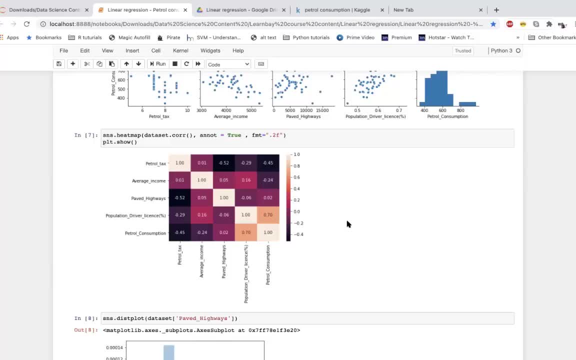 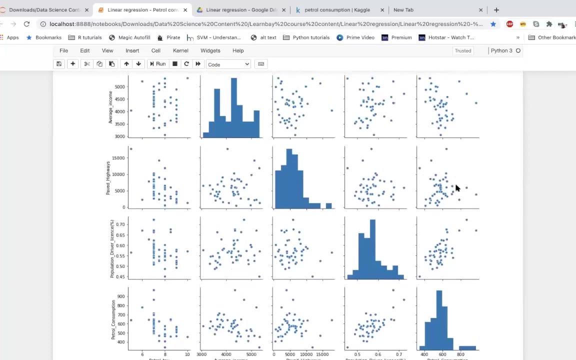 Quite clearly. it's a positive impact, but the impact is so less that I don't really care about it, So I don't care, I don't need to justify it, but I know that. okay, paved highway seems to be a rather insignificant contributor and the scatterplot was actually giving us that sort of indication that you know there isn't much that you can say using paved highways. 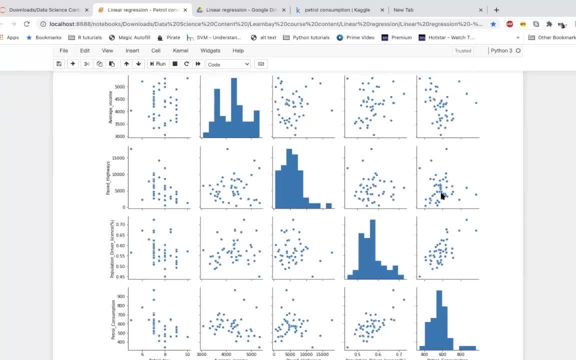 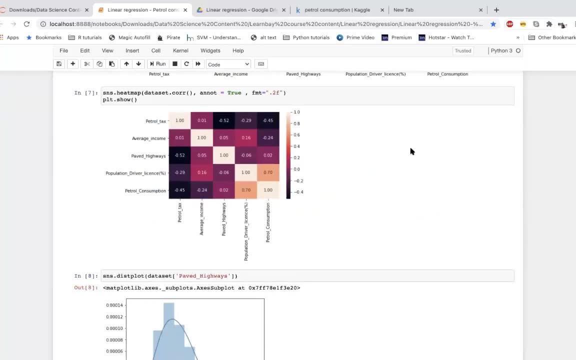 I don't think there's any trend that I can establish for petrol consumption. So that's the other thing. Good, Uh, what about populations, driver license? We expected a positive relationship, a good one, And that's what we have. We've got 0.7, zero. 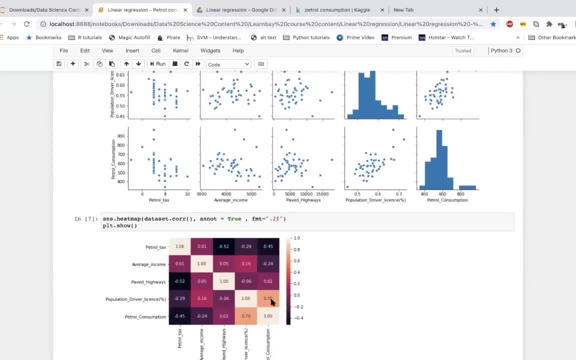 It seems to be the highest correlation that we have. Yeah well, that's brilliant. So, uh, this column quite clearly has a linear relationship, and we'll most likely capture that in the coefficients as well when we actually get this equation. So that's brilliant. 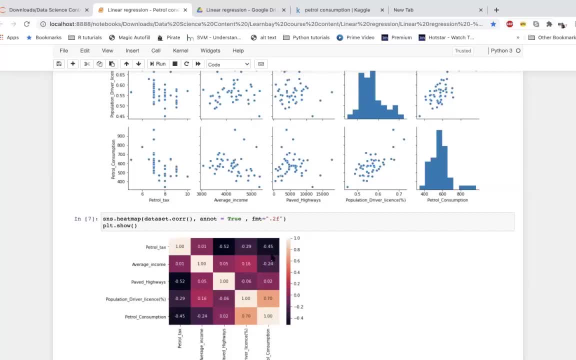 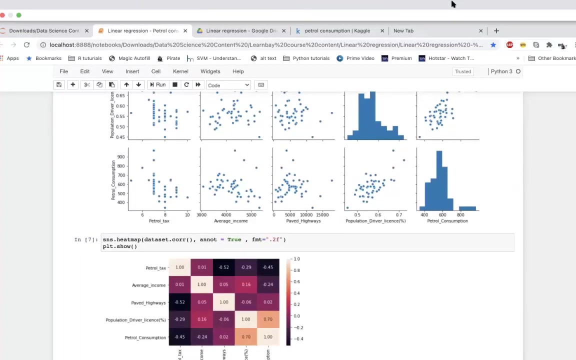 Petrol consumption itself is one good. So, as far as the target variables are concerned, we now understand how each of our independent variables are related to my target variable. My target variable is Continuous- which means that I will be running a regression on this- and I know that some of my independent variables, at least, are contributing, uh, in terms of having a linear relationship with the Y variable, and that's quite clear. 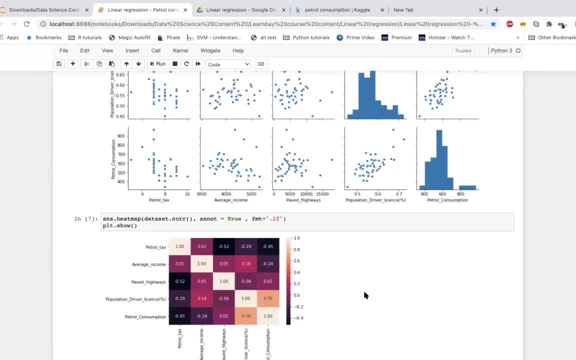 I can see a visible linear pattern, so that's good for us. What else should we check for in this plot? relationship between the dependent variables. So, okay, Uh, highways has a core positive correlation with average income 0.05 and petrol tax 0.05.. 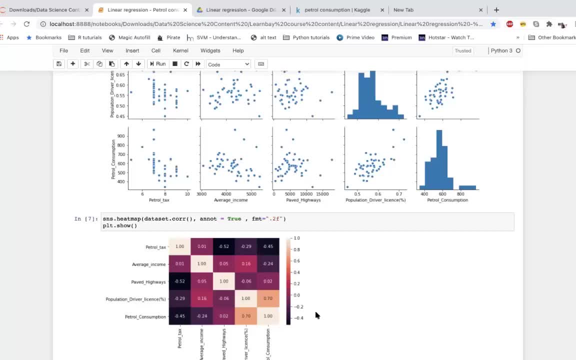 So I mean, when we are building the model for petrol consumption, we have to keep them separate highways, separate from average income and petrol tax. Okay, You're saying, uh, petrol consumption column. Yeah, Third column, If you look at the highways, 0.52.. 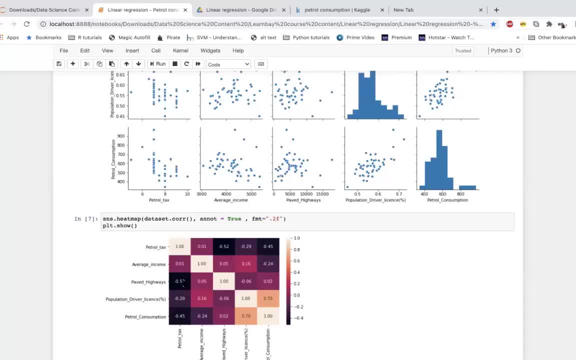 Yeah, So minus 0.52 is the correlation. Yeah, So you're saying that these two independent attributes have strong correlation- negative but strong, which means that you know they can probably cause some sort of multicollinearity problem? 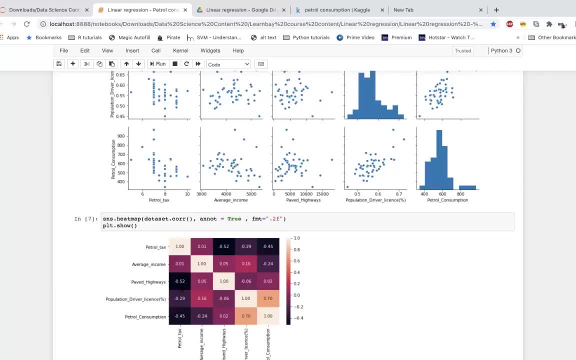 Correct. Yeah, Yeah, Same as with uh, paved highways with average income. 0.05. paved highways and average income: No, but 0.05 is so low that you shouldn't worry about it. Okay, I mean okay. 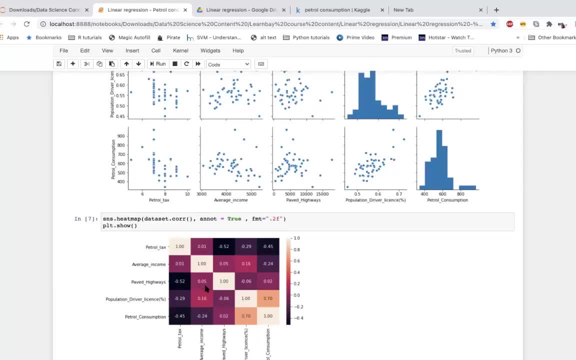 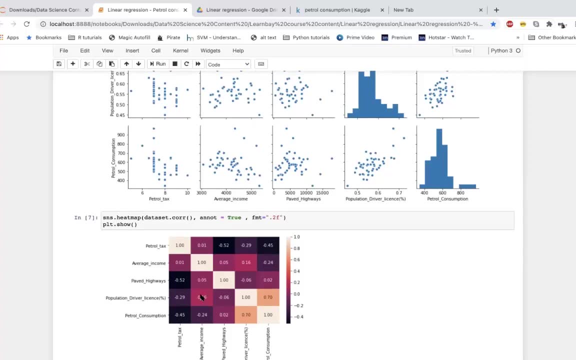 0.05 is in all parameters a weak correlation and you can Not for you about it. So general thumb of rule is 0.5- 0.05.. No, no, Strong old statistical textbooks will tell you: 0 to 0.5 is weak, 0.5 to one is strong on both sides. 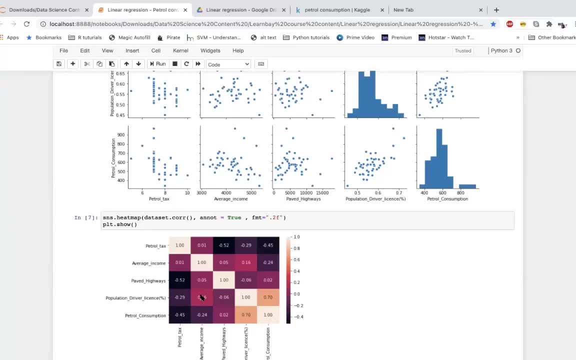 Okay, So 0.5 is the right. but today, these days, you know, people start considering anything beyond 0.25 as significant. They say that weak correlation is up to 0.25. 0.25 to 0.75 is intermediate. beyond 0.25.. 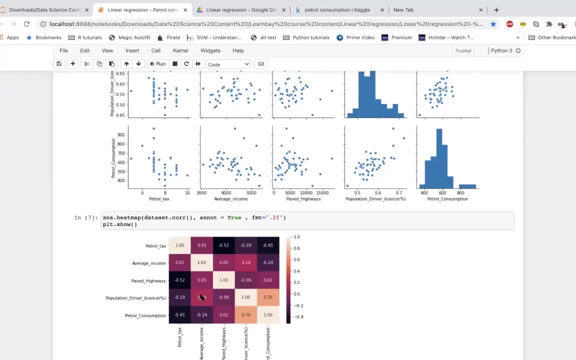 Yeah, Yeah, Yeah, 0.75 is strong, right, Sorry, my mistake. I thought it's: 0 to 0.05 is a weak and 0.5- 0.05 on what you start, That was 0.25. 0.0 0 to 0.25 is weak. 0.25 onwards is considerable, which means that up to 0.75, it's intermediate above 0.75.. 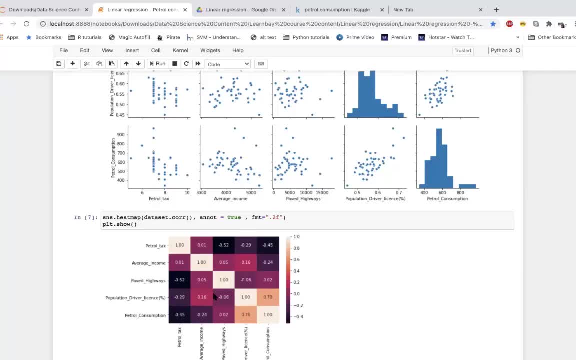 It's strong, Yeah, Yeah. So anything beyond 0.25, 0.3, practically you should not ignore it. You should consider it as- Yeah, You know what do you call it- Significant correlation. So 0.24, I'm still going to ignore without too much worry. 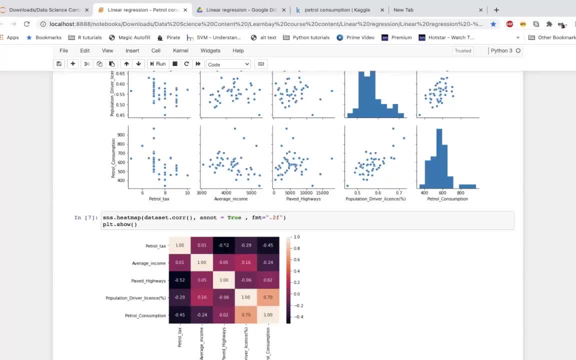 0.16, I'll clearly definitely ignore all of these else. Everything else seems to be insignificant. 0.29 and petrol tax. So again, this could become a problem. This is close to the region where I find it to be a problem. 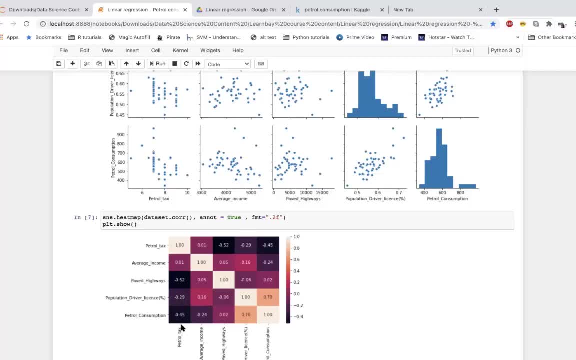 Yeah, It's negative again with petrol tax. So petrol tax seems to be the problematic variable. It seems to be a problem from the looks of it, but I'm not understanding the petrol tax number of driving. if we have no more number of driving licenses, we should expect more consumption, which is the 0.45. if there's more consumption, we should expect more taxation or get a tax rate not taxed by income. 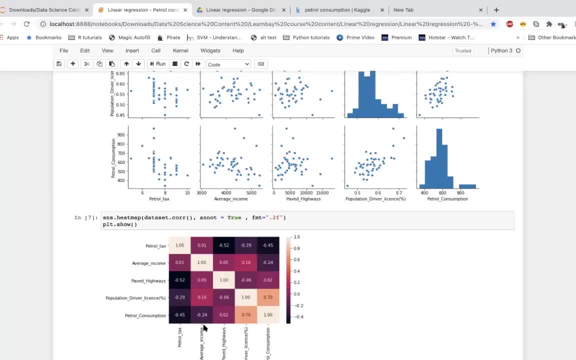 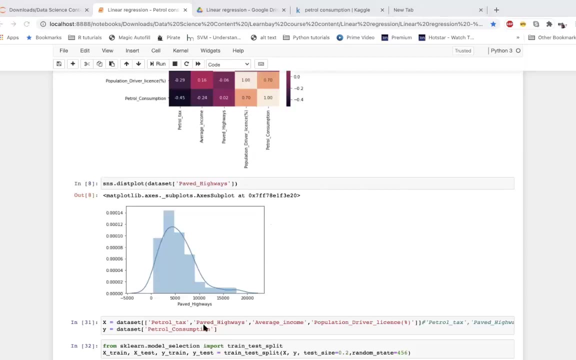 Sorry, Okay, Okay. So we've identified some possibilities, two possibilities which can cause multicollinearity. Let's see what happens. Uh, you know, we'll go ahead For now. we'll see what happens. just a second here. 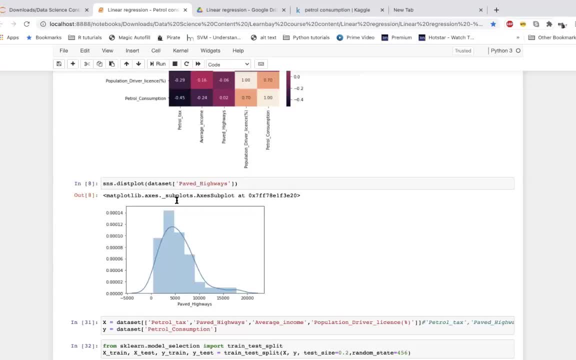 Okay, This is one good way to look at, uh, you know, the distribution for any given continuous variable. This is a curve that will very well represent, uh, the idea that is, uh, you know that this frequency plot is sort of trying to give away. 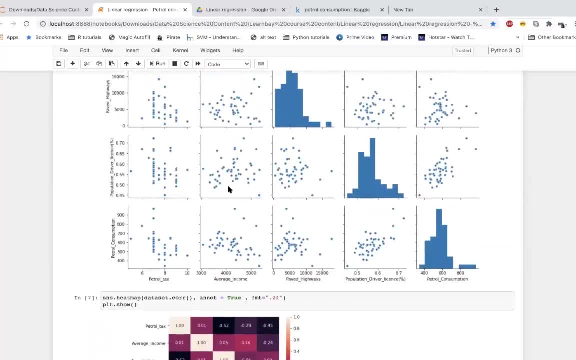 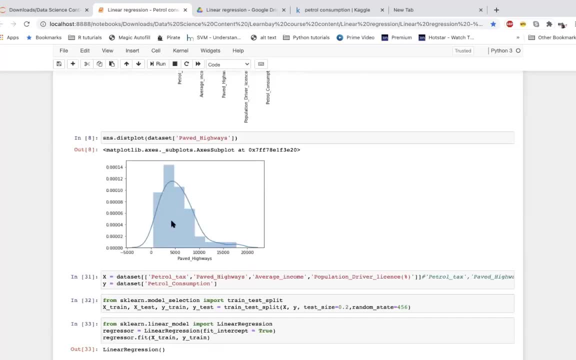 Likewise, you can change these variables and do it for all the other curves Columns as well. So let's say this: paved highways, paved highways. What kind of a distribution would you call this? Almost normal, almost normal, Actually, paved highway seems to be pretty normal. 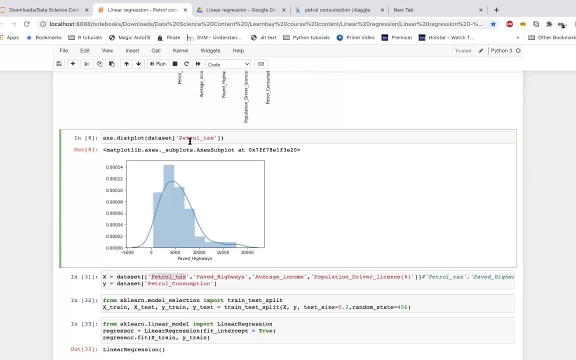 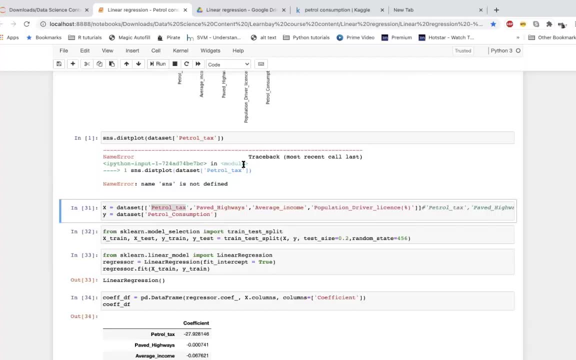 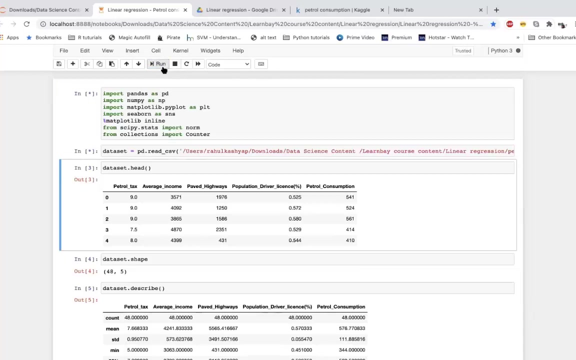 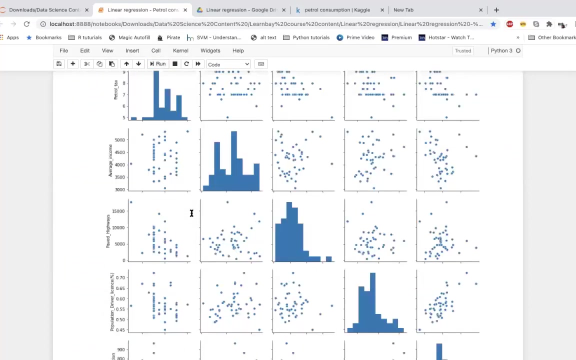 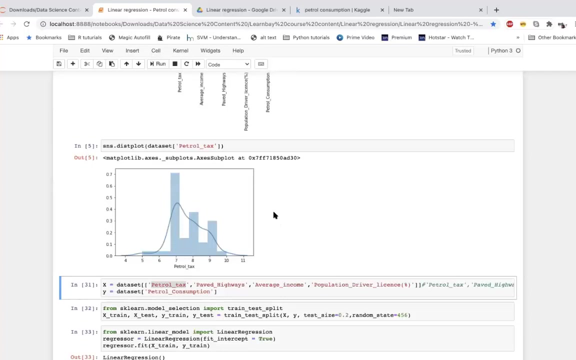 A little bit of a right skew, you would say, but not so much. I mean, it looks very normal, But you have to be careful if you're going to Natural. The total tax seems to be a very fluctuating sort of distribution. 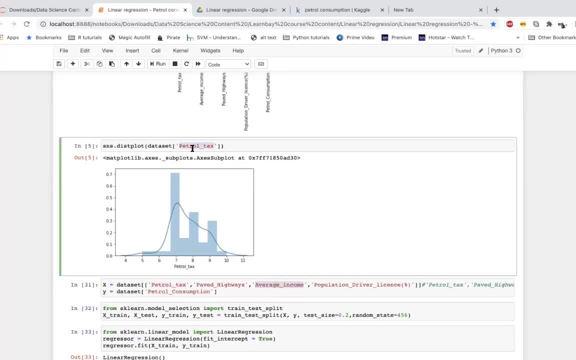 you know, known distribution looks like average income is also almost, yet again close, but I wouldn't say normal, but it's quite close to normal actually. in fact, in some scenarios I would be happy to accept this as normal. but distribution plot is a good way to. 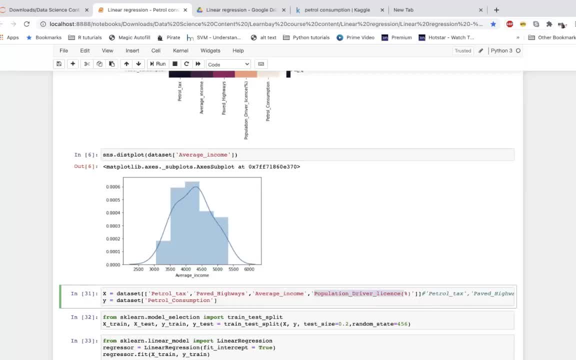 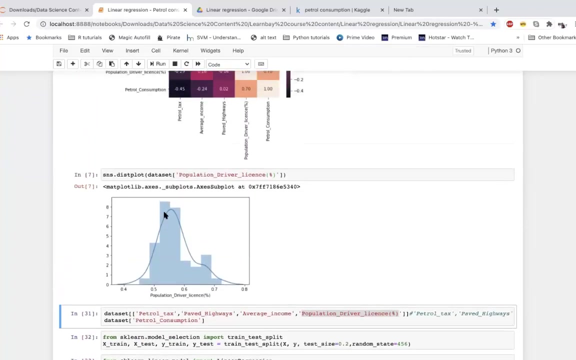 visualize your data. well, trying to understand what the inherent distribution is. we have since seen that can help with missing values and everything too. so again, this is also quite good. seems close to normal, actually. this distribution so looks close to normal. Raul on the y axis. 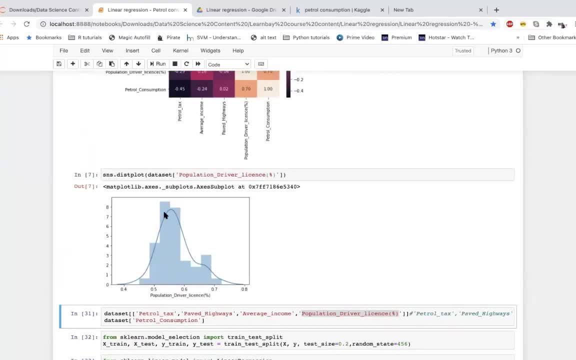 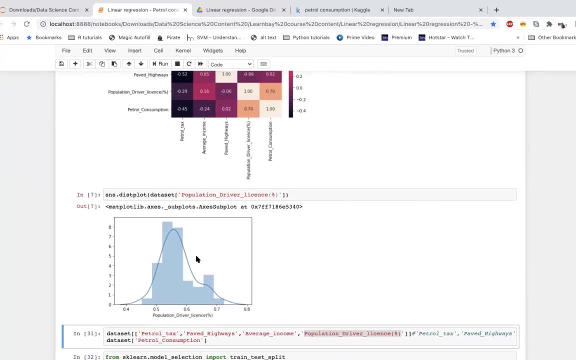 can we have the distribution values on the left hand side actual histogram count for this curve? If you can populate the curve, I mean the population, this mean probability on the height, and will it that be of any use? Because I mean we'll. 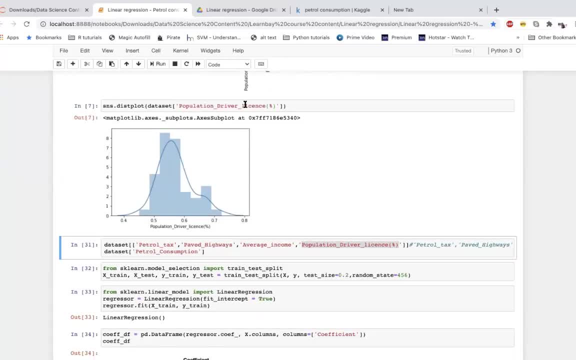 get to know what is it. Yeah, so that can also be done. Maybe you have to change a few parameters here, No problem. Yeah, That can also be done easily, because it's simply a relative frequency. it will become. that becomes a. 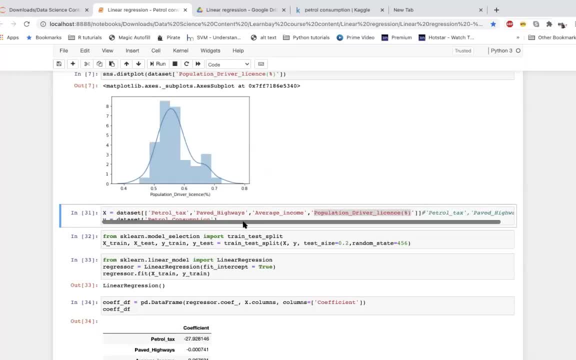 percentage. Okay, so now let's move on to do the actual analysis, where we will try and build a linear regression model over this data. we have some sense of what to expect out of this, So what we're doing is we're breaking it up into two. 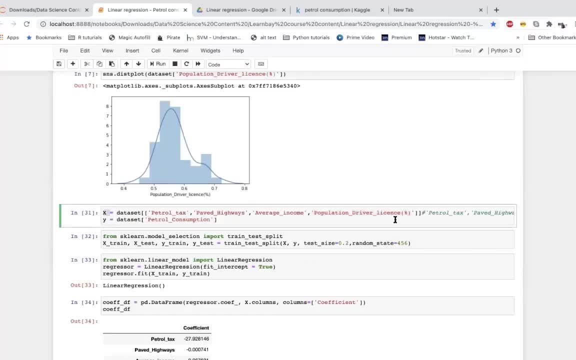 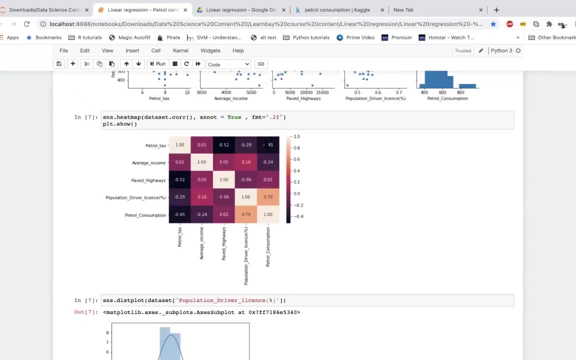 data frames. One is for x, which is, which has these four independent attributes, the four attributes that we're going to work with, Although we know that your paved highways does not seem to have a significant contribution. 0.02 is very low. Rest, all I'm willing to consider are: 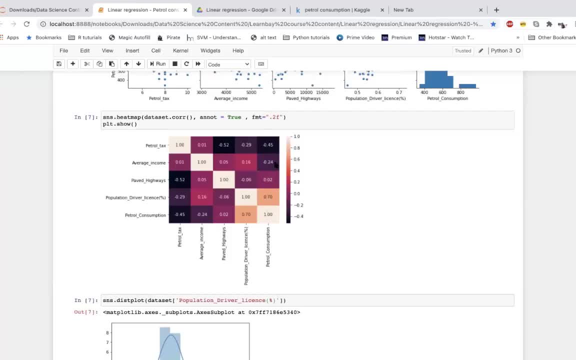 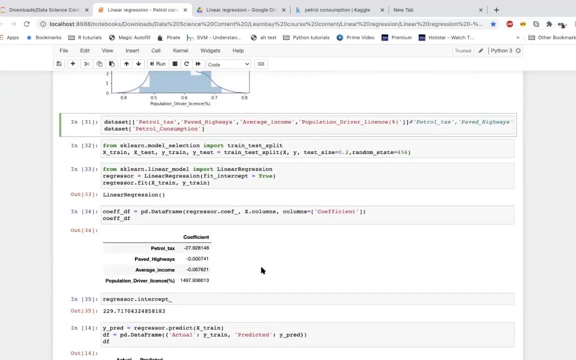 significant. Point two, four is a little dicey but I'm still going to be okay with it, But paved highways is very low, So paved highways does not seem to, you know, be important, but it could be, so we're not going to tamper with it, we'll keep all. 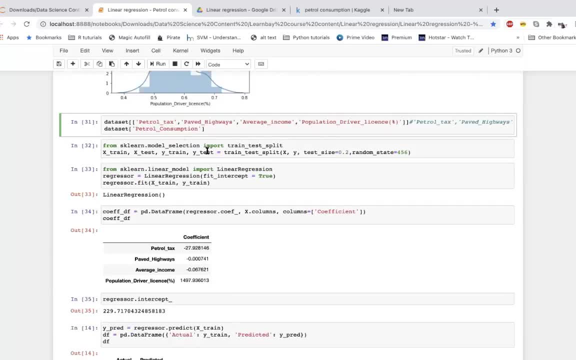 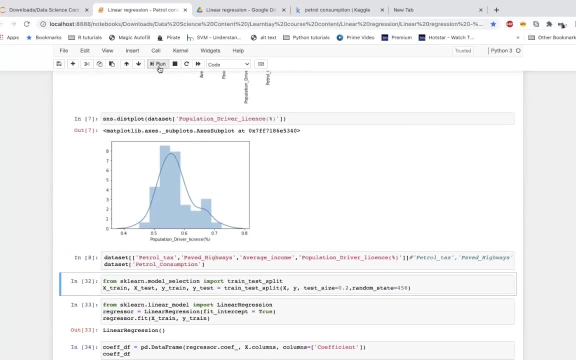 the variables right now And we'll keep the Y column separate. So I have one question. Sorry for digressing a bit, because I use some pipeline. It's because of which I get some additional insights as well when I run for these data sets. So one question: what I wanted. 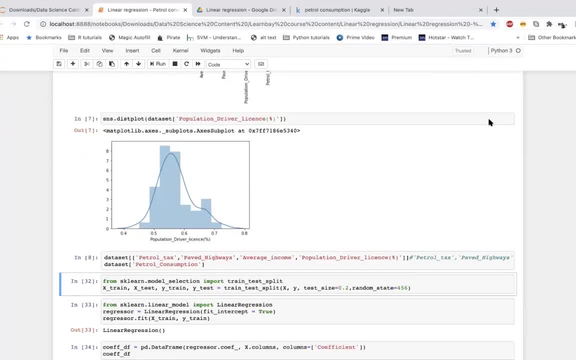 to ask is: will you be also covering on the vif variance inflation factor to identify the? not right now, not right now, actually somewhere down the line we can. but vif as a measure, for I can, just you know, just for you to be able to use it, you just need to know. 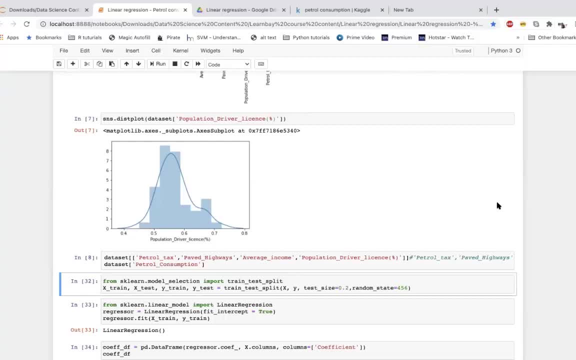 that that vif should be somewhere up to five, six, seven, five. any vif greater than five indicates that multiple- yes, multiple- reality exists in the data. So that is just another test that you can conduct. So I typically don't, you know go. 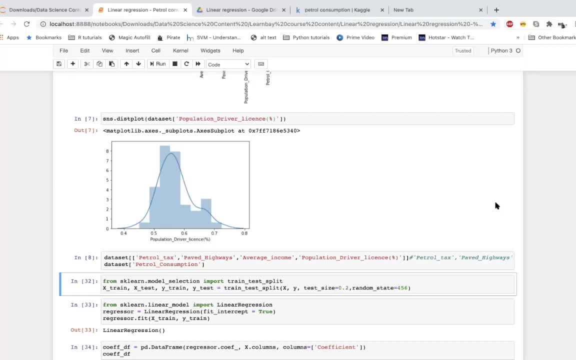 that route. Okay, okay, Because I got some mixed insight when you, when you go with that route, the paved highway has the lowest vif compared to any other point. If the lowest vif, so yeah, okay, And the other which has high vf. 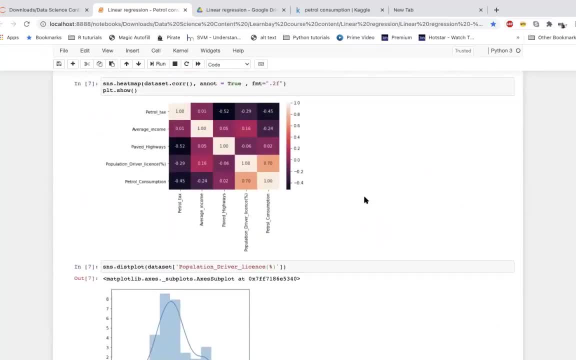 in fact the one that, yes, petrol tax, as well as one second. let me open it out Including the population driver license that has the highest populations driver license. Okay, so we have a sort of mix up between petrol tax, paved highways and population driver. 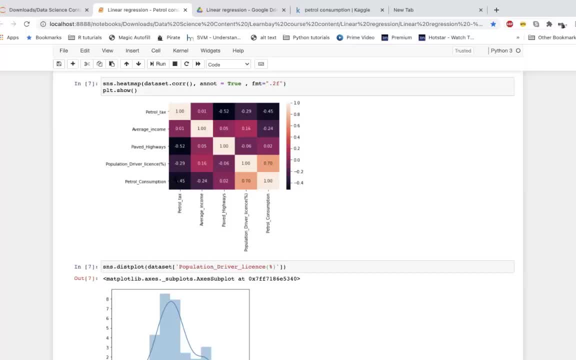 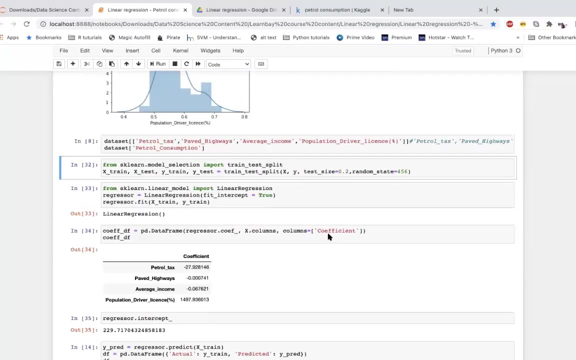 license. Yes, these are the columns that are causing problems for us. These are the ones out of which populations driver license is giving you higher vif? Yes, Okay, I think we don't. So I don't generally do that discussion. You guys can read up on it And we can discuss. 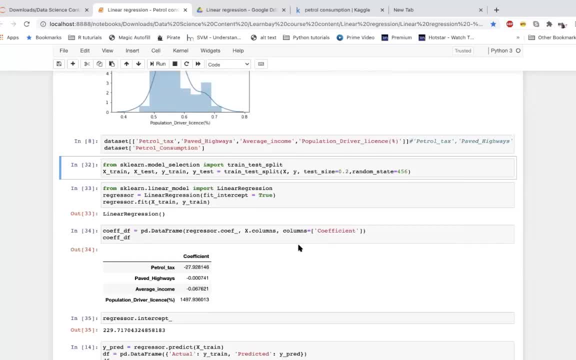 it, maybe in the next class if you want to. That is one way of checking for multicolinearity. The thing is, the reason why I don't discuss it is because, see, these statistical models have these limitations, where we want to worry about things like auto. 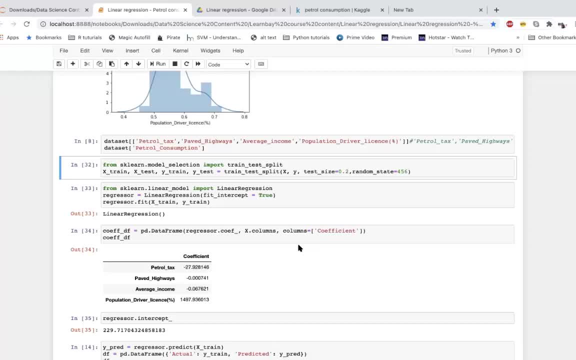 correlation or multicolinearity, And we are starting off with these simplistic models. But as we go forward you will realize that most of the regression that you do you'll mostly be using nonlinear models. for that, And inside nonlinear models, you're mostly using machine learning approaches. 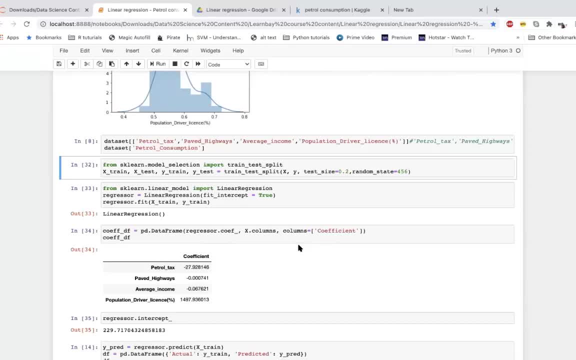 which means that none of these assumptions need to be checked for. So there are so many other ways of doing these regression problems where you don't need to worry about multicolinearity or autocorrelation. So at the end of the day, everybody skips. 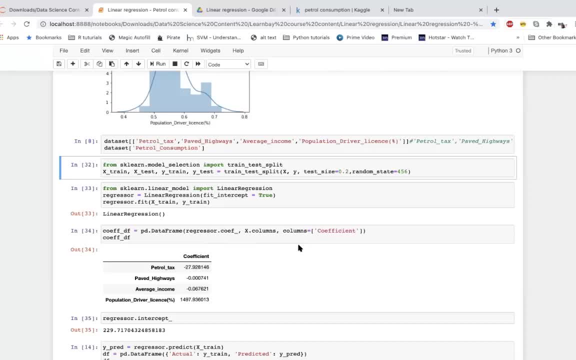 this part And when he's actually implementing it, he's only using machine learning approaches where there are no assumptions, which means that there are no limitations. So there's no constraints, nothing. There's nothing that you have to check, nothing that you have to ensure And all approaches. 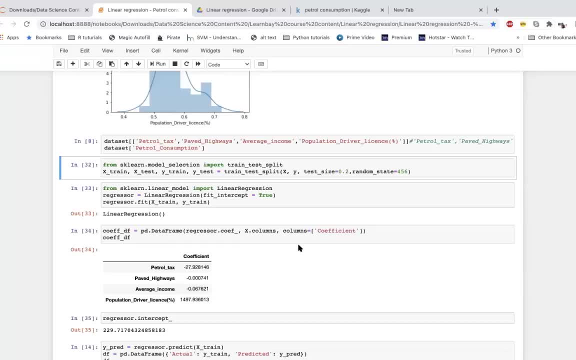 work on all kinds of data sets, So we will generally skip this over. So, in fact, if we get into the details of statistical tests, there's so many statistical tests, almost everything. we are going to cover five, six tests inside the. 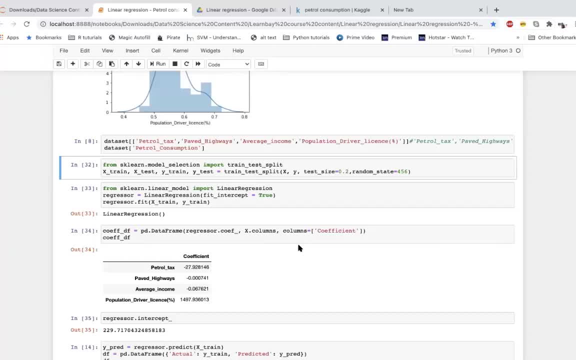 stats model implementation. That's why I choose to do the stat model implementation, so that we can discuss a few hypothesis tests along the way. Then this one: multicolinearity is not a problem. If you're having a multicolinearity problem, you better go with a. 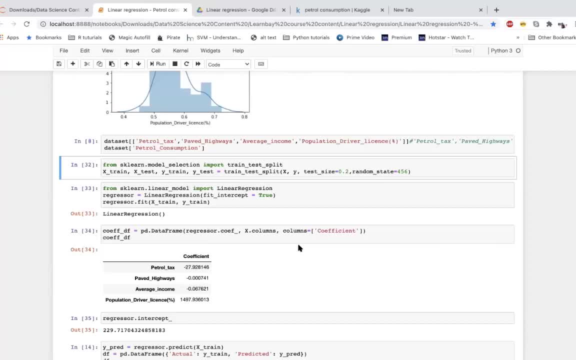 nonlinear model. See, the problem is with larger data sets, you always have multicolinearity. no matter what you do, The moment you have data sets that have more than 15, 20, 25 attributes, there'll always be attributes that are related to each other. 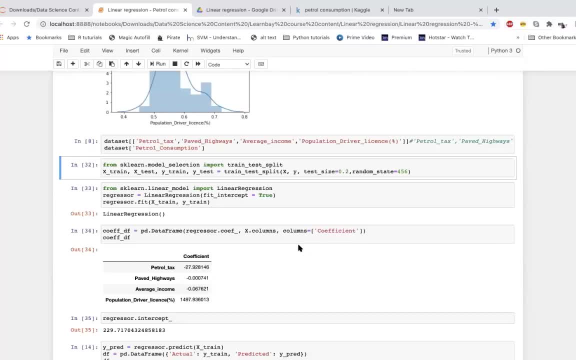 Yes, you have a. you have things like how many years you've been in the company and what is your years of experience in total. Generally, these numbers are correlated to each other, So you will always the more number of features you have in any 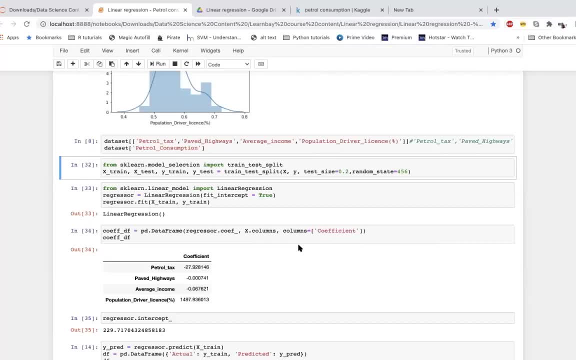 model any data set, there will definitely be multicolinearity, which means that the moment that happens, you'll have to start hacking and chopping, removing variables from your analysis, for you to be able to run the statistical models, which is why everyone just immediately switches over to machine. 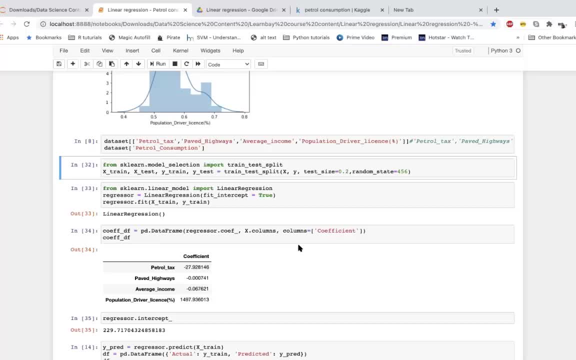 learning approaches which can very well ingest all the 30, 40, 50, 100, 500, any number of variables that you pass to them and churn out a result without you have to worry. worry about anything, You know you. you don't have to look at these correlation plots. 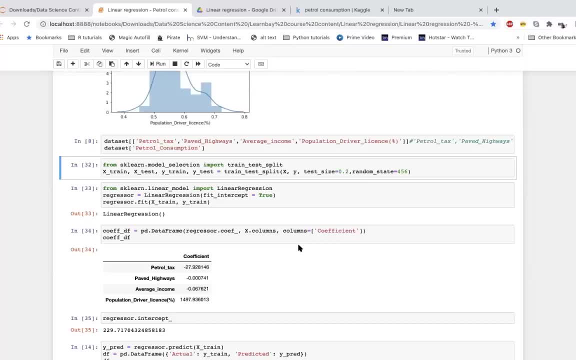 You don't have to look at all possible combinations of those 500 attributes where there are multicollinearity problems. what you don't have to care about any of that because those approaches are so easy and still give you so good results that inevitably you're going to switch. 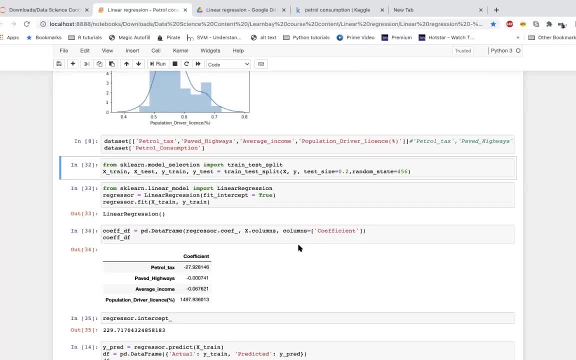 to. that Makes sense. I mean, that's been my observation so far. Yeah, I think it's clearly aligned what you're explaining. That's what generally people do, but if you're interested you can let me know and we can discuss it maybe. 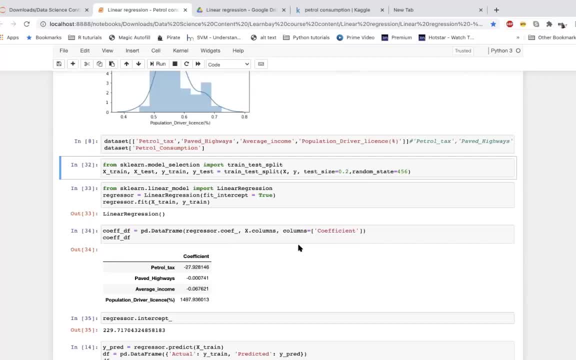 sometime. Sure, Yeah, It's a just. it's just a little bit of math. 15 minutes per discussion. I just want to. don't want to go there right now, All right, But we've identified the possibility of multicollinearity in our case. 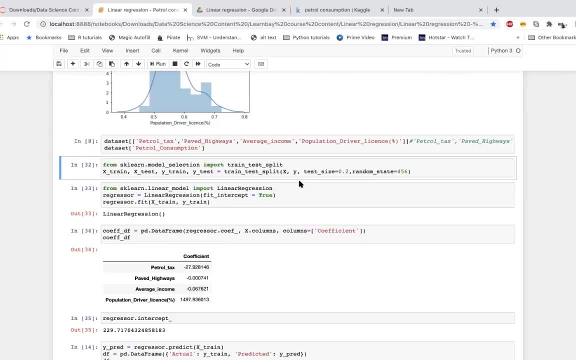 And I've told you about two typical ways in which you know a severe multicollinearity problem will manifest. So we always check in our models whether something like that is happening or not. We'll see what happens in this case, But for now 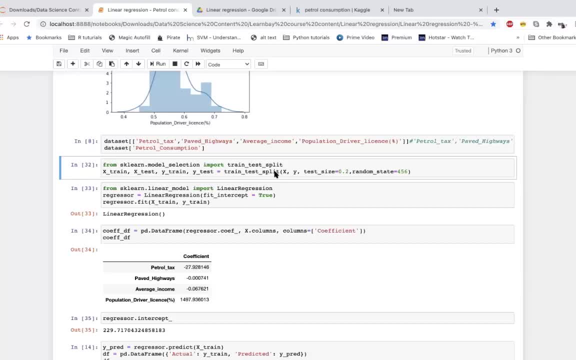 we'll. we'll just move on and start. begin begin with the model building exercise. Now, this model building exercise starts off at one point. for all models, no matter which one we are doing, It starts off with an initial breaking up of the entire data set. 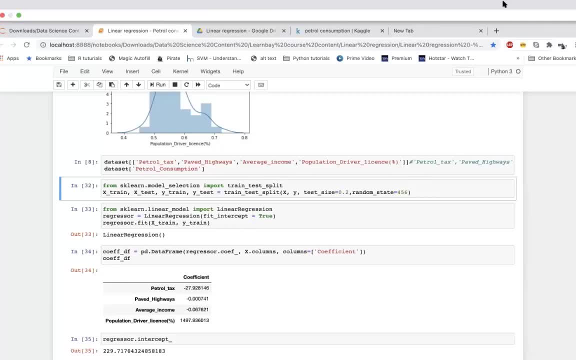 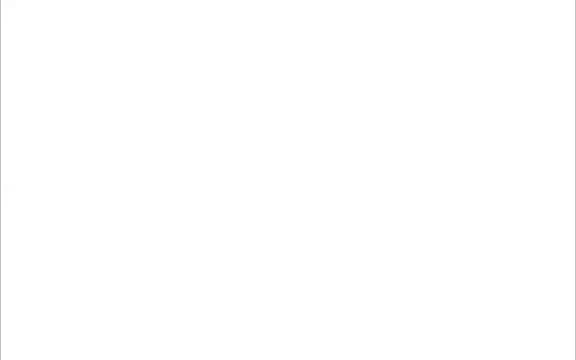 So what you do is you've got a data set to work with. You break that up into two parts. So what happens is: so you have a data set. Now you've got to train a model. You will train a model. What's the purpose of building any model? 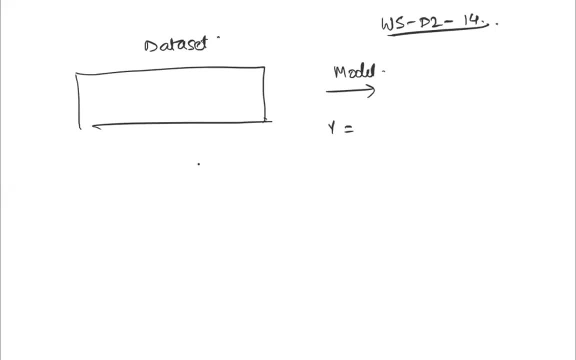 The purpose of building any model is to create a functional form like this: Y is equal to X one, X two, up to X K, which later on, when you have new values for X one, X two, X K, you can put that value into the model and the model gives you a value for Y. 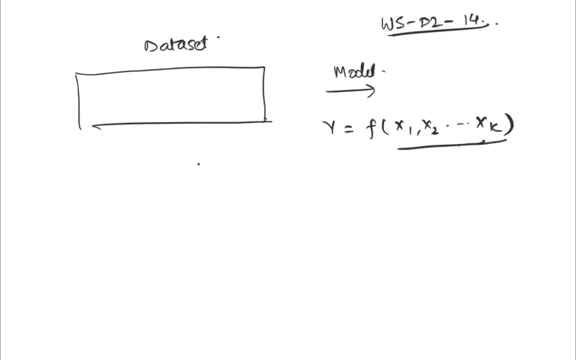 That's the purpose of me building any model, which means that the purpose of looking at any historical data, looking at any data that you already have, to be able to build a model like this. it requires the model to be able to perform well on any new data that it sees. 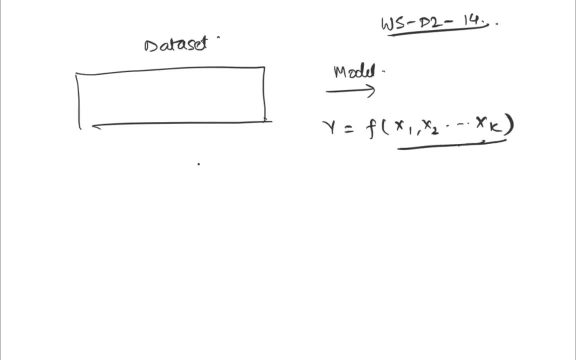 Well on any new data that it sees. it requires the model to perform well on any new data that it sees. This concept, there's a term for it. It's called generalizability. What is generalizability? Let's say you've got a hundred rows of data. 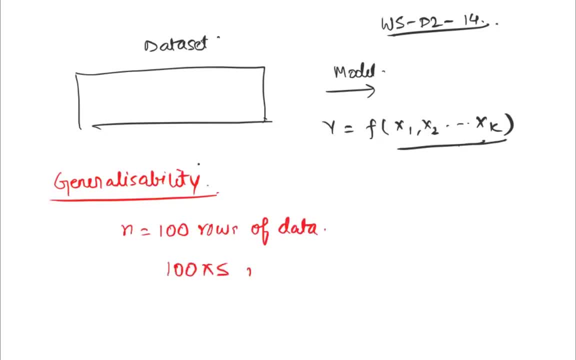 So you've got a hundred cross five matrix. So there are five columns, out of which four are independent, Five are uh, one is uh dependent. You have a hundred rows of data. You build a model over all the hundred rows. 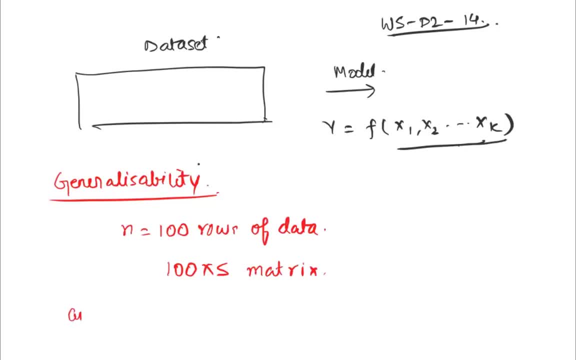 You build a model over all the hundred rows. Now, any new row, your model should perform just as it, just well as it performs on these hundred rows. So you can build a model and you can then check the accuracy of the model. The model will not be a hundred percent accurate, because you cannot create a 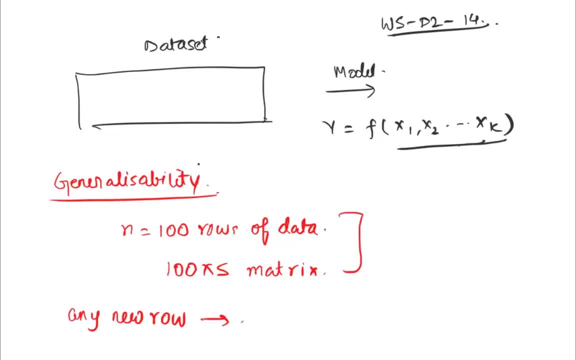 line that will be able to pass through all hundred points, So you'll have some error. So let's say you have 10% error. This error is called training error, The error that you get on the data set upon which the model has been trained. 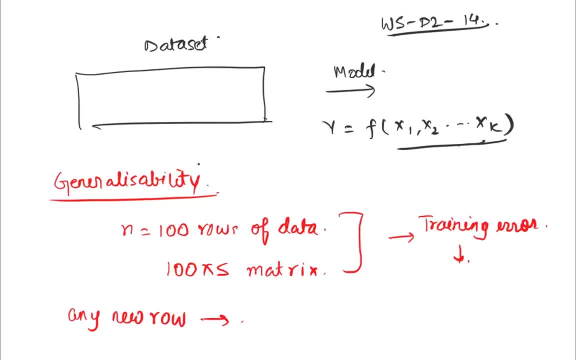 Let's say you had a hundred rows. You use all the hundred rows to train a model. The model gets trained on it. Now the model has some training error on those hundred rows. Let's say some. let's say it is 10% now for any new rule. 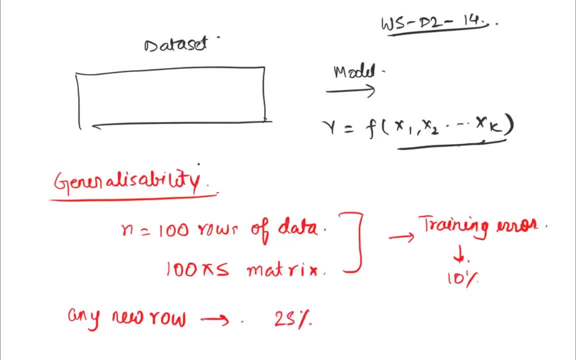 If suddenly your error becomes 25%, then you immediately know that your model was not generalizable. If you get an error in the range of, let's say, 12% or 8% or 13%, if you're getting errors that are close to 10%, 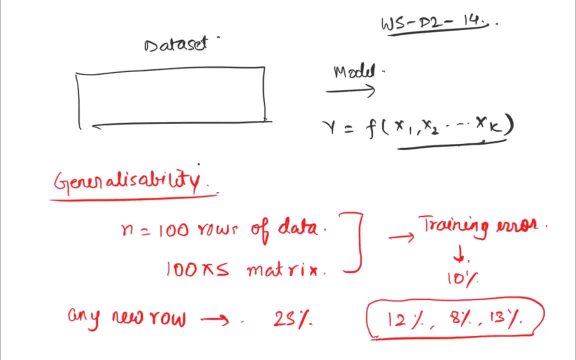 you are okay. You say that. yes, on new data, my model is not doing as well, maybe in the case of 12 or 13%, but still it's doing comparatively as well as it did in the data that it was trained upon. 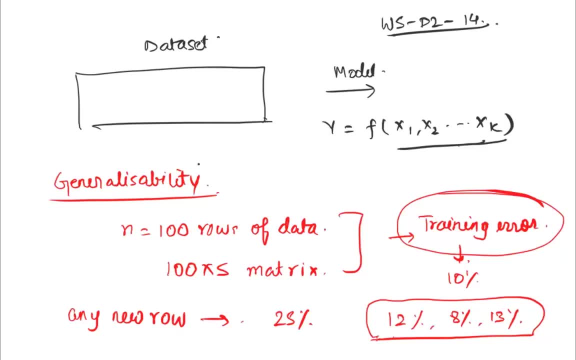 Such a concept is called the concept of generalizability, which means that the model does just as well on new data as it does on the data that it is trained upon. Now, why are these two data sets different? because the new data. the model has never seen the training data. 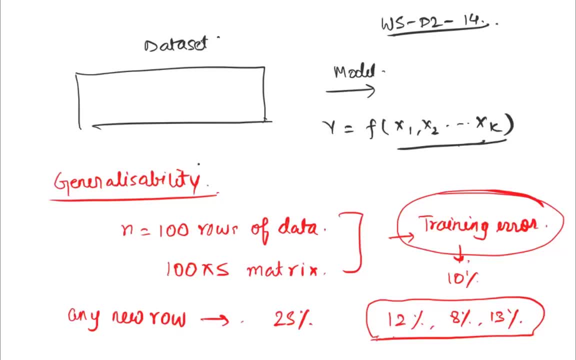 The model has seen. model has seen that for this combination of X one, X two and X three, you get this much Y. based on a hundred such observations. It has created a model and now it is predicting based on that model. But the idea of generalizability, 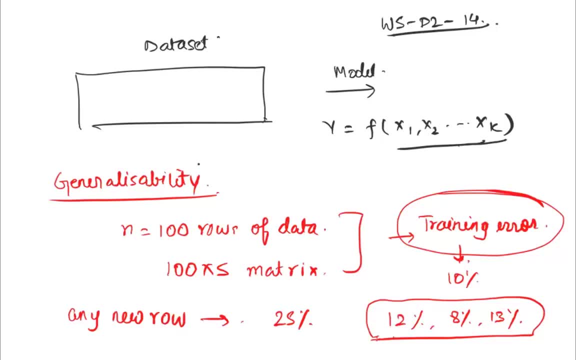 generalizability requires such models to do just as well on new data as they do on data that was trained upon, The simple reason for that being the purpose of building a predictive model is to be able to predict when you actually do not know what the answer is. 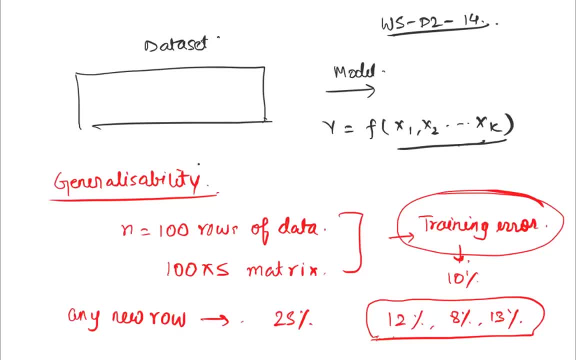 When you do that, that is when it's actually useful. when you are able to say that, okay, this is the expected sales in the next quarter, That is when you are able to plan for it, but there's no way of actually knowing what the actual sales is. 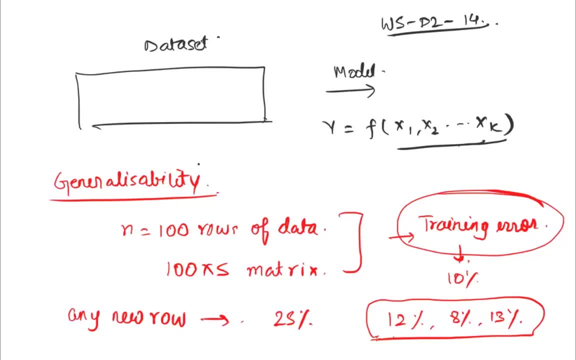 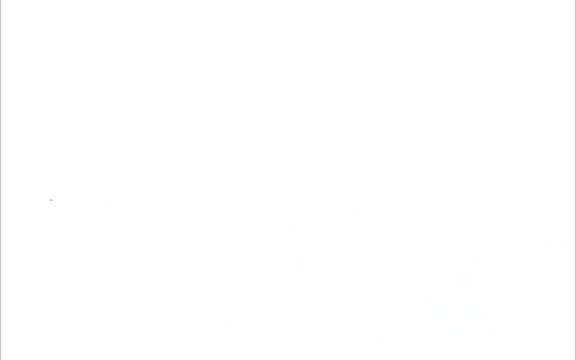 So it is in those scenarios that this is important. So the model, the model, should be able to perform well on new data, And that is the idea of generalizability. Now, in that direction, there's a process that has been set up to ensure that your models are. 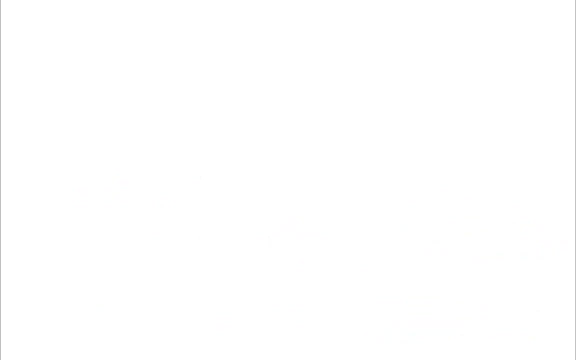 generalizability: to ensure that your models are generalizable. What's that approach? That approach is the approach of doing a train test split. What is this? You've got your data. You break these data into two parts, You keep 70 to 80% of the data and you call it train data. 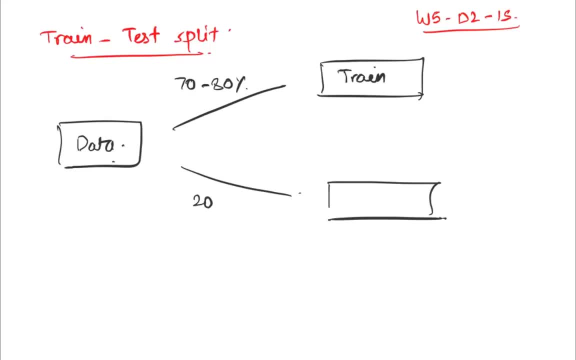 The rest of the 20 to 30% of the data is called the test split And these data are called train data, And these data are called train data is called the test data. what this means is on these, on this 70 to 80 percent of the model, 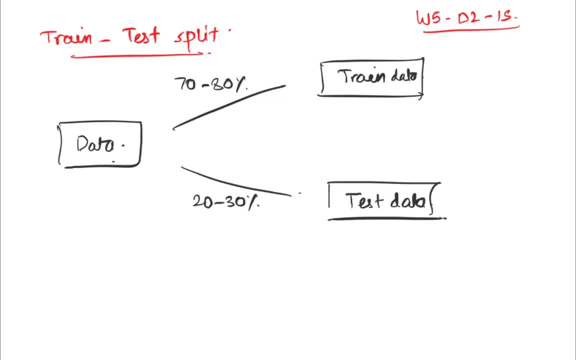 you will train your model, you will pass this to the model, to the model function, and the function will basically use that 80 percent of the information to build a model, that model you will use. this is data that you have taken out. the test data has been taken out. it's only this: 70 to 80. 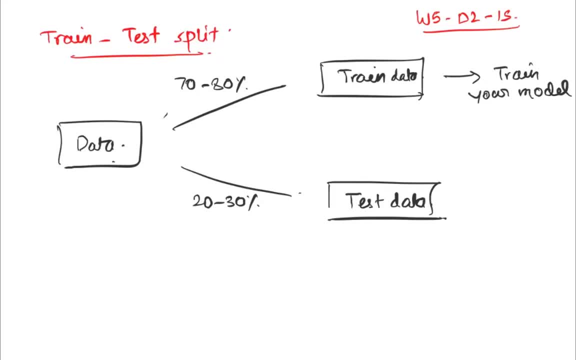 percent, which the model is seeing while it is getting trained. now this model will perform predictions on the test data- data that it has never seen. it was part of the total data set that you got, but you've broken up in, broken it up in the beginning and you're using a large part. 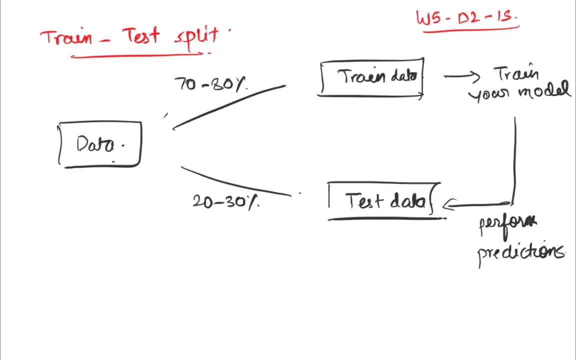 of the data set that you got and you're using a large part of the data set that you got and you're training and the small part that is left which the model has not seen, that part you're using to actually see the accuracy of the model. so you're looking at. 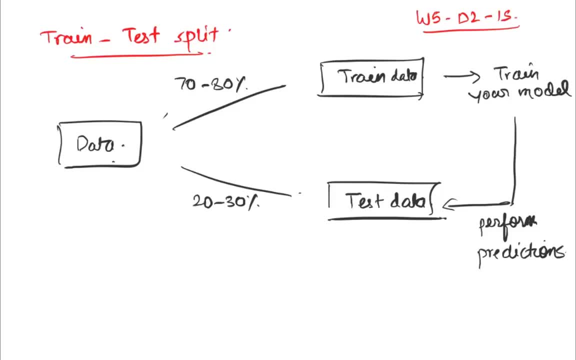 so what do you do then? you then look at, you train your model, you use that model to perform predictions on test data. as a result, you get test accuracy. you already have training accuracy when you train your model. you then predict with the model on train data and you find out the 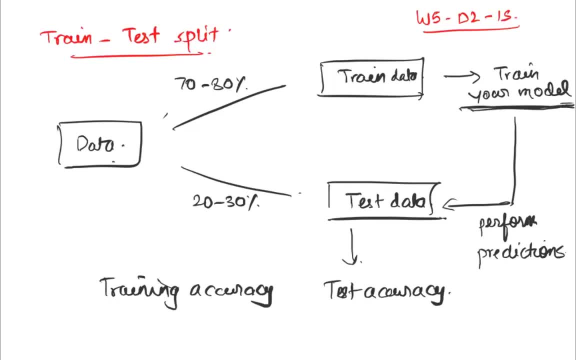 accuracy. accuracy is found out by the matrix that we used: mse, rmsc, ma2. those metrics are used to find the accuracy of the model. you now have two accuracies. you've got accuracy on some 20 or 30 of the data that was separated, not passed to the model while it was getting trained, and 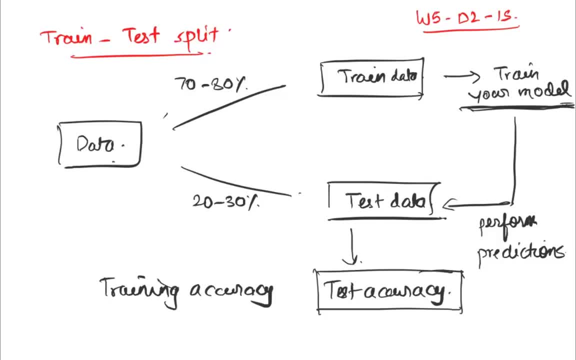 then you've got the difference. but the difference is that this method has already been used many times until now. started, but when the major bulk of the data and the model was trained on this and you have looked at the accuracy. if these accuracies are, 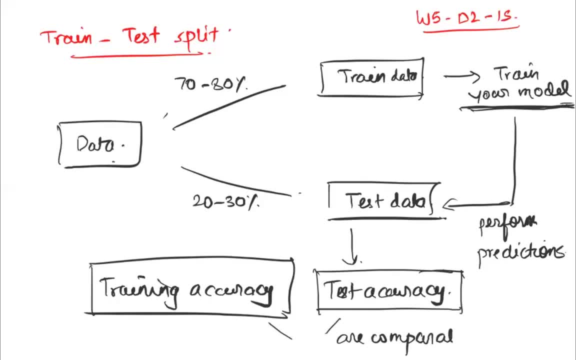 comparable, Then this is a generalizable model And you would be willing to accept it as long as the errors are low. if they have comparable accuracies, but those comparable accuracies are 20%, then you don't like those models. But if you have comparable accuracies like 84% and 83%, then 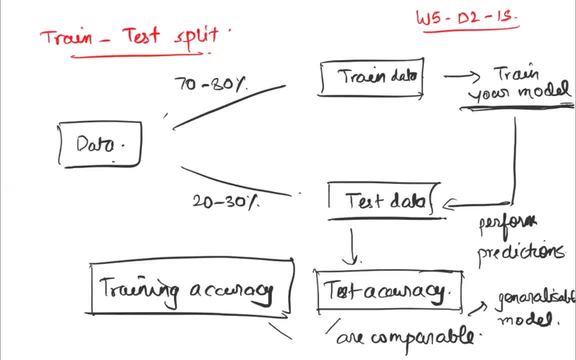 you'd be happy to accept a model like that, where your test and train accuracies are similar. The simple idea here is to be able to ensure generalizability with whatever data you have. You do not rely on any new scenarios to be able to check whether. 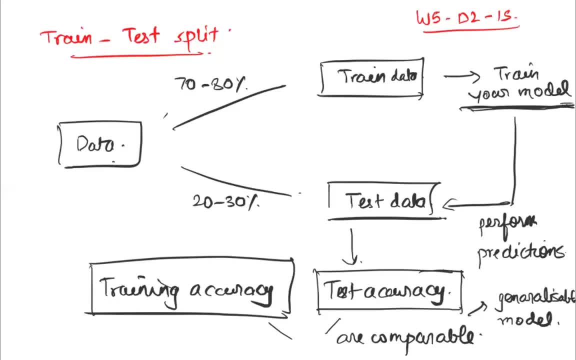 your model is generalizable or not. Whatever data you have, you use 80% of that data to train your model And the rest of the 20% you use to check whether that model you have trained is generalizable or not. Does this make sense? 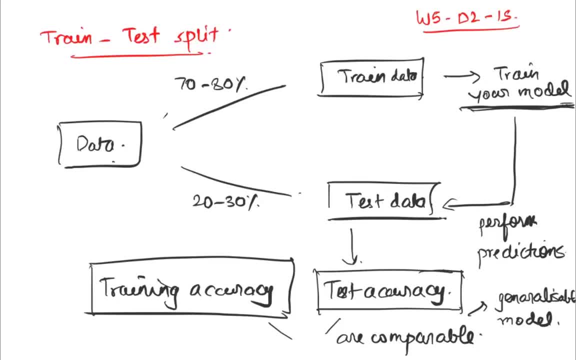 And how do you check generalizability? You see whether your training accuracies and testing accuracies are comparable or not. If they're comparable, then it's called a, then it's a generalizable model, which means that no overfitting has happened. 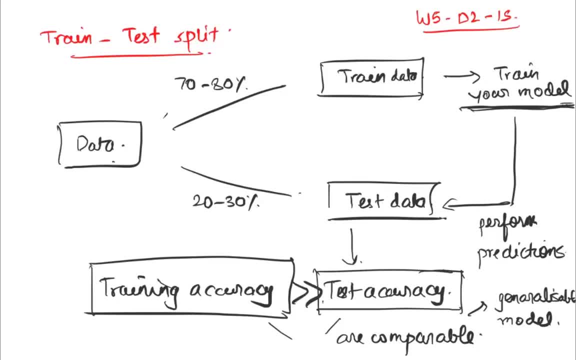 It's not. if your training accuracy is way more than test accuracy, That is a clear indication of overfitting, That your model has overfitted the data. If your train and test accuracies are comparable or similar in a close range, then you are happy. 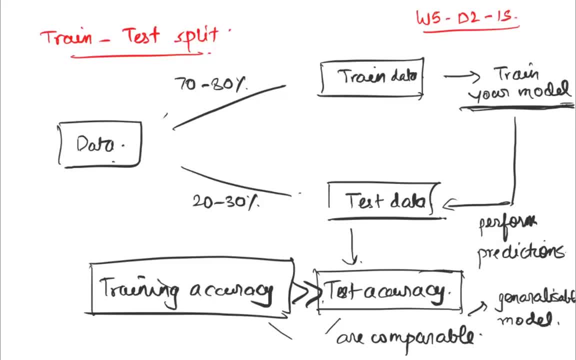 You say that you've got a generalizable model. The kind of accuracy that you're getting on train data is similar to the kind of accuracy that you're getting on test data. Is this idea clear? Yes, sir, And when it talk of 7080 train data and 2030 test data, do we I? 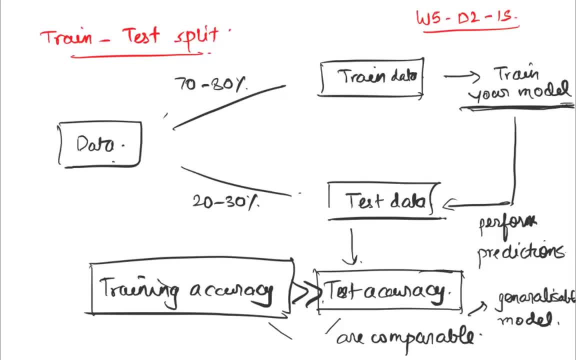 mean, do we cleanse the data beforehand or do we just take their audit and just trade? Do you divide them into change it and test data? And maybe I'll do that. We just do a random sample and randomly pick 80% of the data. 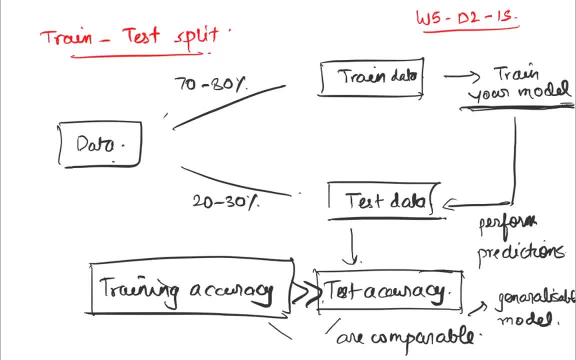 What is left becomes the test, Okay, And on that 70 to 80 to train the model, I might know, decide to remove outright, etc. etc. So already, data pre-processing has already happened. right now, Whatever data you have, you're going to use it for model building. 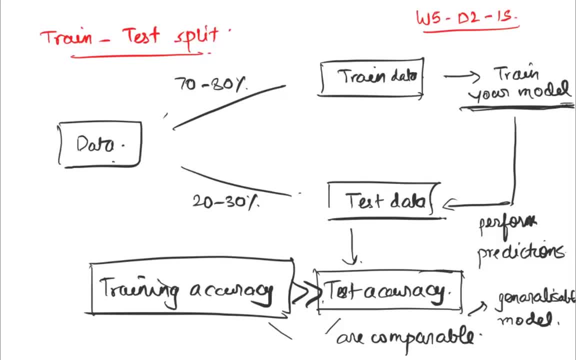 which means that you have 48 rows. So you will put 80% of those rows for Training and 20% of those rows for testing. So pre-processing will happen on 20 to 30 and or as well like 100%. 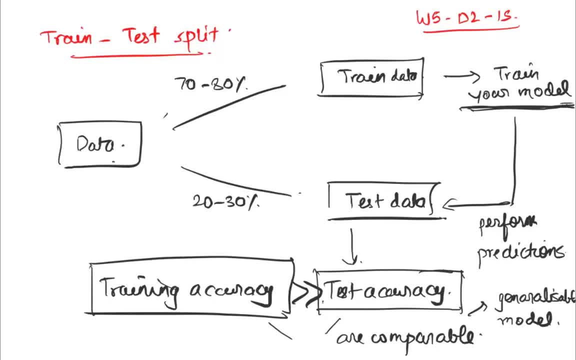 of the entire data. Anything that you do before this has to happen with the entire data. See, whatever format you are going to create your model, that is the format in which you need your test input. So you know, manipulation you're doing with data has also to be. 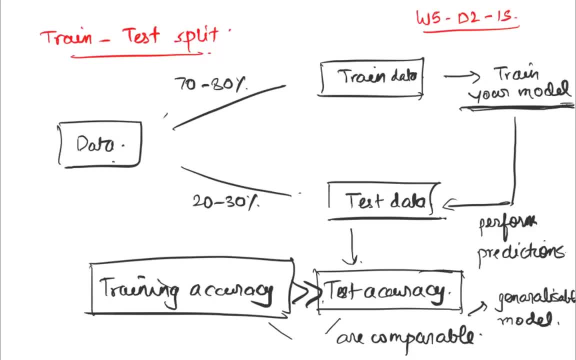 done with test. That is why we do this break right at the end of EDA and data pre-processing. Once you pre-process your data, your data is ready for Analysis, Then you do that split, Then it's in that case. 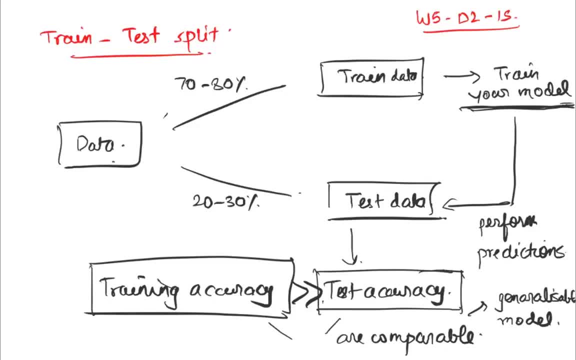 It's high, very highly likely that 20 to 30% would fit into what this, the rest of the side to date- is trained to. So yeah, that should be fair. I mean, sometimes we can take the different approach as well as is. 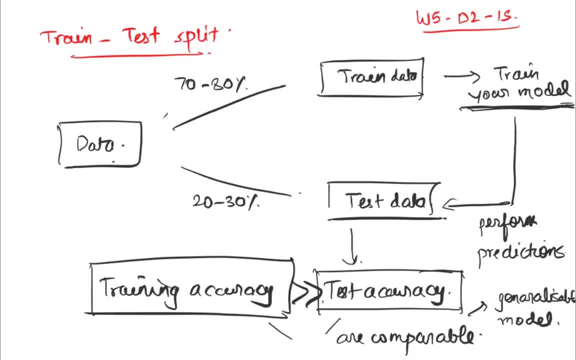 thinking it's that a different approach. I mean that you just random select the data- 70 to 80, you know, cleanse it and then 20 to 30 leave it as it is. I don't do any cleansing- and then, once you train the data, 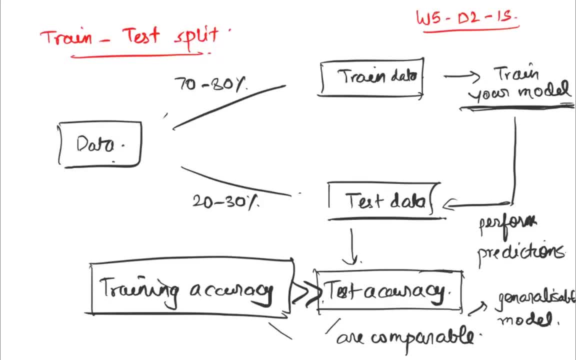 You will then test it. test it on the 20 to 30.. The only problem with that is that the nature of data in both scenarios should be claimed. So if you're using, instead of looking at, daily sales, if you're using average sales as an input in the independent, in the training, 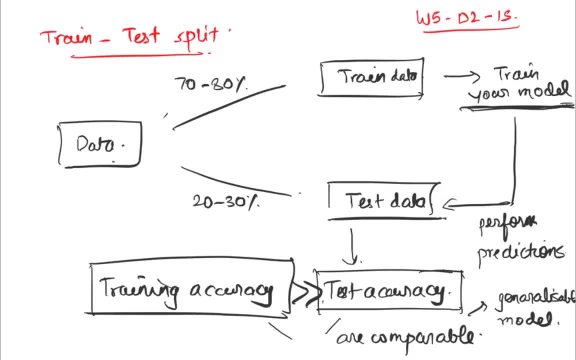 then that is what the nature of the data should be, while testing also right, Right, You're doing it, train, You should do it, test also, which is why this thing needs to happen right before you build your model. Okay, I was not talking about the attributes, are talking about the data. 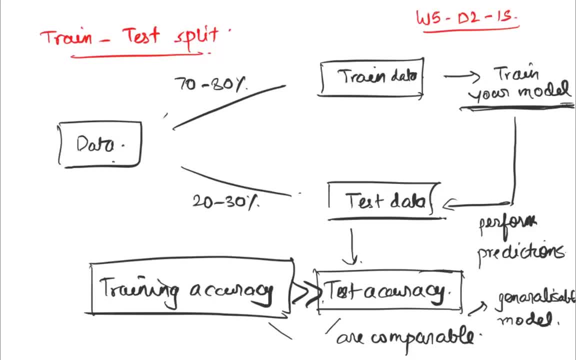 points. It's in the attributes cleansing part. So imputations, Yeah, Yeah, Yeah, but still you should maintain integrity. Yeah, you do your data processing and everything, and then, before building your model, you break it up into train and test. 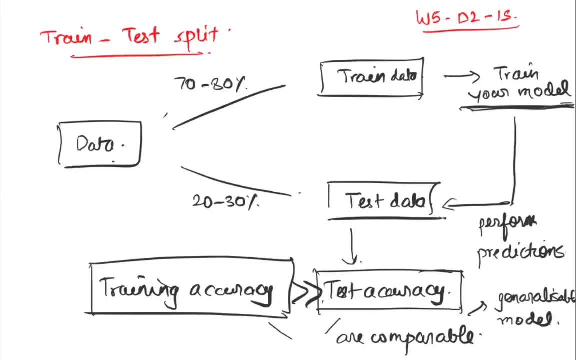 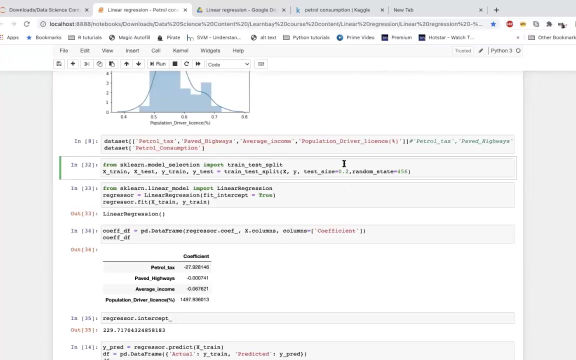 Okay, get it All right. Okay, this, this part actually does that: the importing a train test split function, which is present inside a scalar model selection, and we are going to pass a few, a simple parameter to it which says test size is 0.2,. 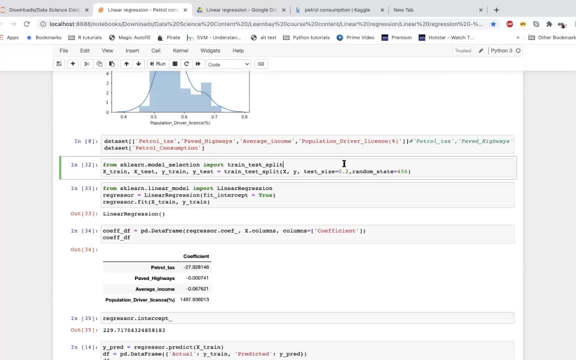 which means that I want to use 20% of my data for testing and I assign a parameter called random state is equal to 456.. This is a question for you. Find out what random state this argument does. How will you find this out? 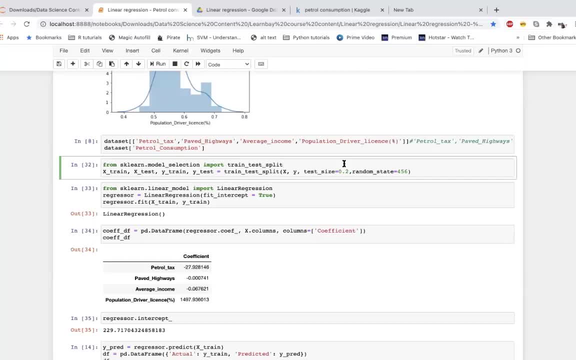 It's like the sample seed, right? So every time, Yeah, it's like seed. If you've used R before, you'll remember it seed. Yeah, For others you can try and explore. I say: if somebody asks you a question like this, how will you explore this? 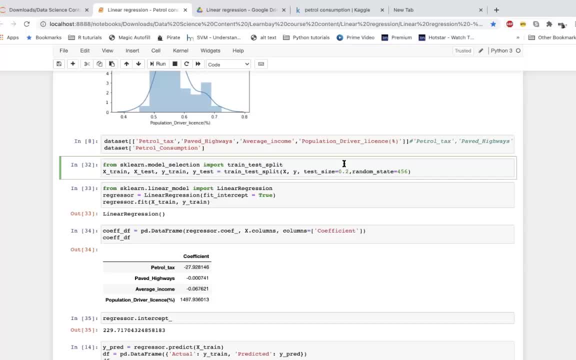 Geek for geeks, Geeks for geeks. Yeah, Okay, Go for it. I can Go for the method: train dir, train test, split and check it out. What does it all these? Yeah, go to the documentation. Always try to go to the documentation. 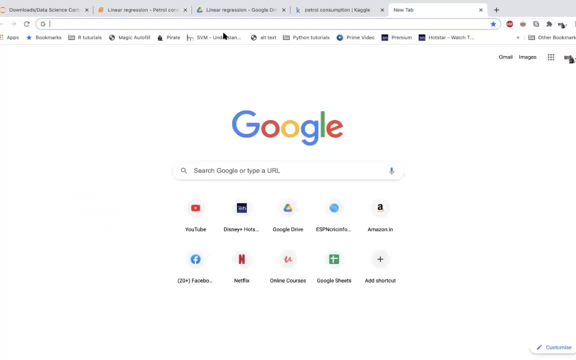 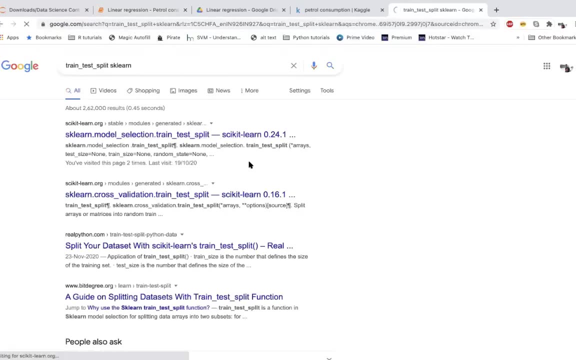 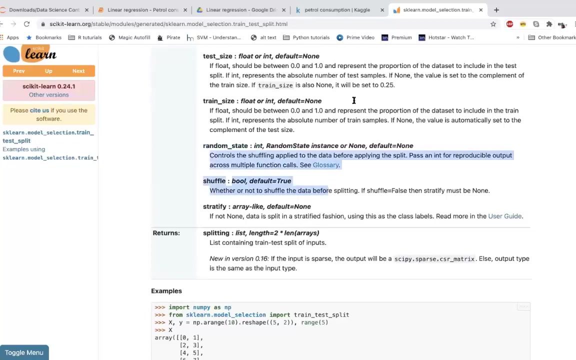 First, just you know, and if I don't get anything, yeah, Google skill and go inside that method. you know that that method will have a description. Yeah, it's always good to see the documentation. Yeah, go to the documentation safest, and that the reason. 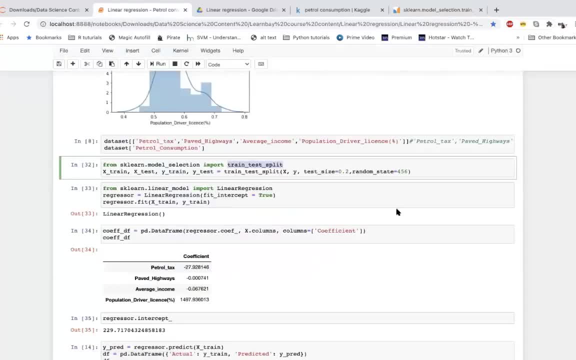 I say safest is because it's important. You know, a lot of places have some random explanations for stuff And even even after that, Geek for Geek for the implementation and use. Yeah, those are good. Yeah, it will give you some nice examples, examples that will help you understand it. 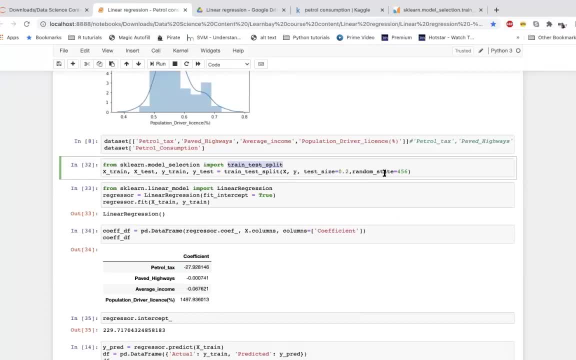 Yeah, and I've said you read about it. It's a simple thing. It's an important thing, though, especially, especially when you're working in a business environment, in a work environment- you're not when you're not doing personal work. So try to figure it out what it is, and actually, let's start. 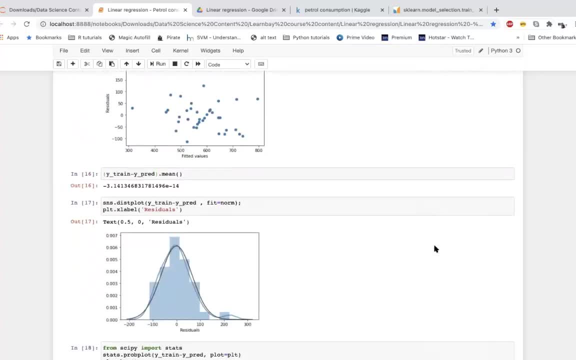 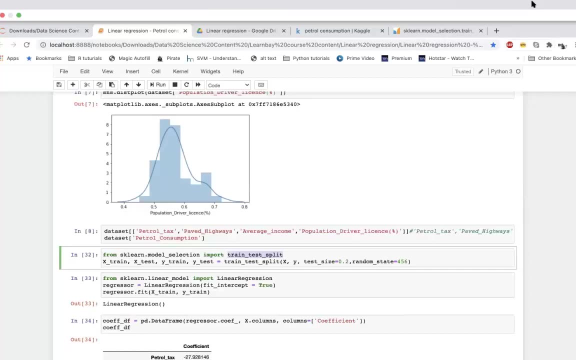 Stop at here. I wanted to, you know, get off with this linear model. Unfortunately, no, this will give us some time for the next week to know the test and rule, So we can- it'll be next week more effective, Yeah. 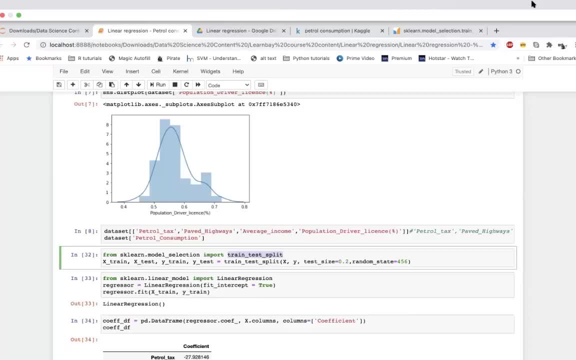 Anyways, we've done a lot of discussion today, Also yesterday and today's class has been a lot of discussion time. Go to see: these codes are relatively intuitive. You should be able to understand. if you want to go a little further, go ahead with it. 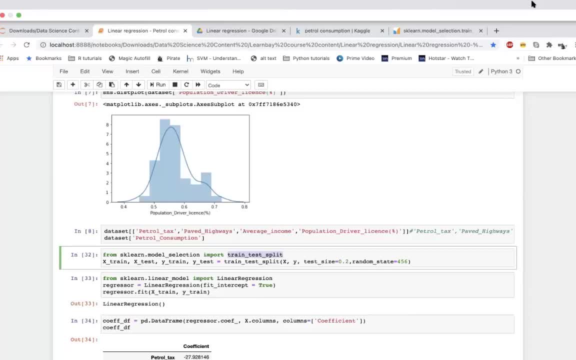 but definitely try and consolidate from a theoretical point of view Everything that we've learned for linear regression. The whole idea of you started off with modeling. See, this is. these are first steps. in some time We'll be at a point where, in one day, we'll finish the theory and the case for a algorithm. 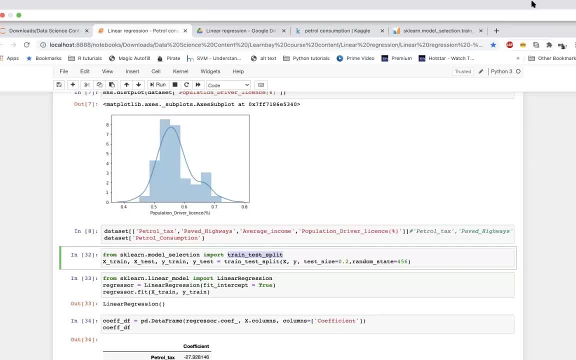 This is the best time, you know, and we are trying to let it all sink in, So try to read as much as possible at this point. These are relatively simpler topics to read upon. This should also help you, you know- get a feel of what this whole modeling thing is about. 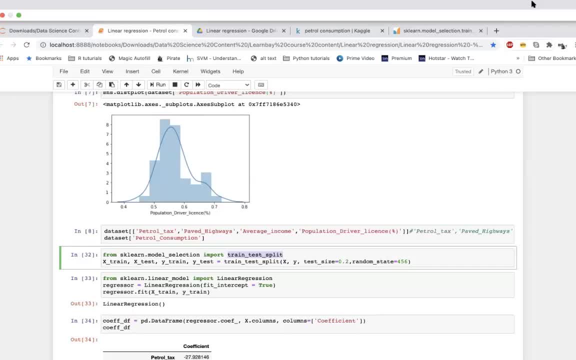 We'll try and do. we will get to more complex data sets, But but right, although what we've chosen are important data sets, These data sets are important because they help me bring out certain things or certain areas of this analysis that are important. 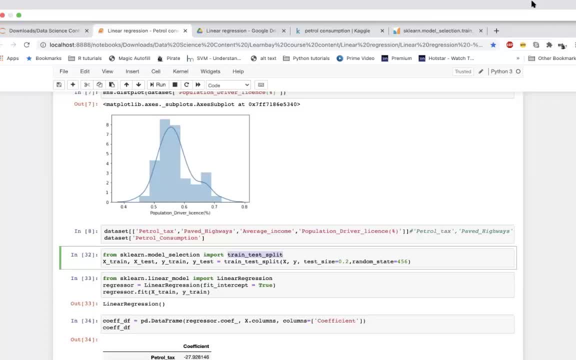 which I would otherwise not be able to bring out. So all of these red sets have their own importance. This might look like a small data set, but this will help us think about things that are important. So try and consolidate everything that we've learned. 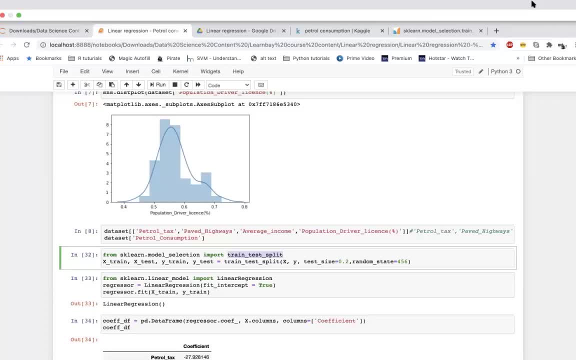 I think let's stop for today and come back Speak. Yeah, Yeah, Okay. So we have done correlation check, right, And we are done this catapult like a fair plot. So we're interested in some points, Okay, And but we're not considerate. 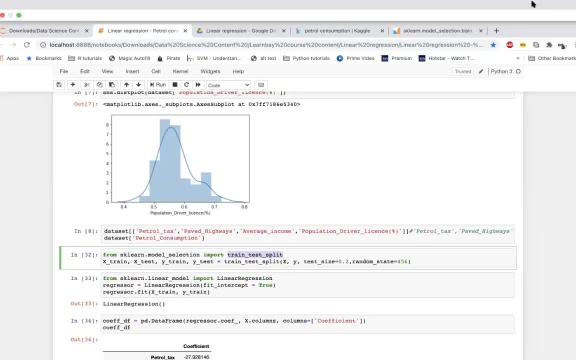 We are passing all the columns Okay, into all the variables to the model. Okay, The analysis is only for understanding or like no mandatory. We have to do this. Yeah, Got your point. I understand what your problem is. Your problem is that. 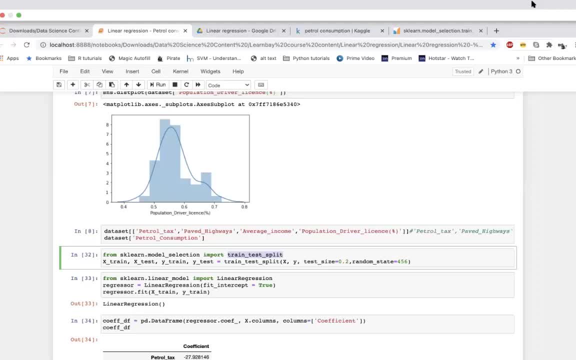 When we were doing our analysis. we were making it seem like the most important thing at that point And we were trying to understand as much as possible. Same was the case when we were doing it for Titanic And I understand your frustration in seeing that. when we started off the modeling, 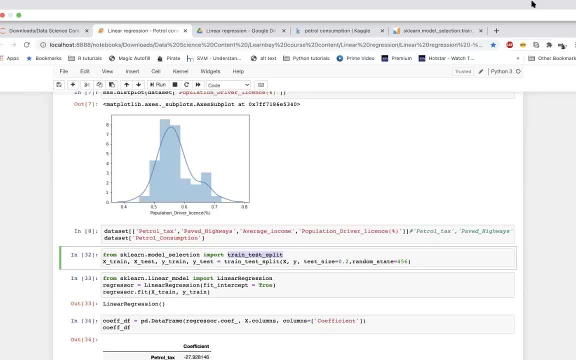 we were completely agnostic of what we'd learned back then. So, even though we knew that paved highways, let's say, does not have a significance in your contribution, We are happy to keep it in the list of variables that we've created a data frame for. 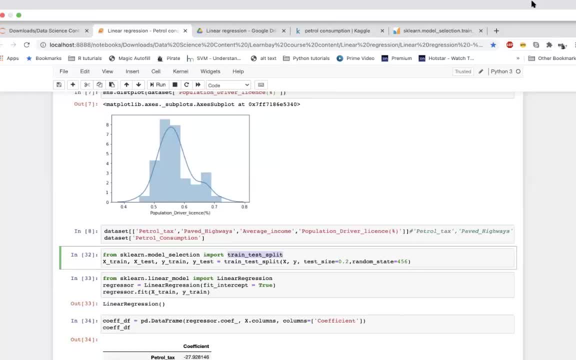 That's your question, right? Yes, sir, Yeah. So the answer to that question is, see, that exploratory analysis has its value, but the value is not in making what you call absolute judgment about what certain characteristics of certain models could be like. 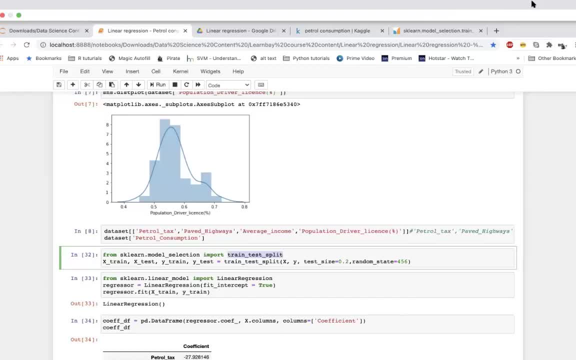 We know that linear models bring out, you know, linear relationships between variables And one way to find that relationship is to look at correlations. But you know, in actual modeling exercises, when you've got not one variable but multiple variables to work with, 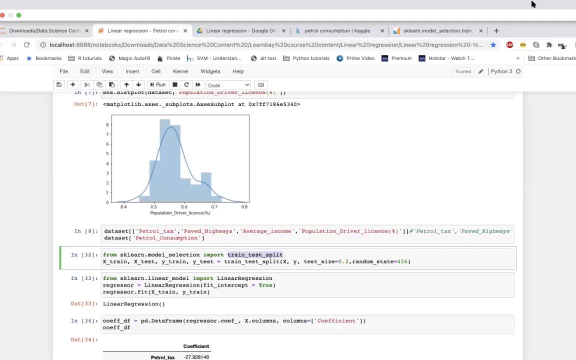 sometimes you will not be able to visualize relationships that models can actually capture. So it's not a good idea that just by doing you know preliminary exploratory analysis that is biased in some way, because you know if you're doing correlation. 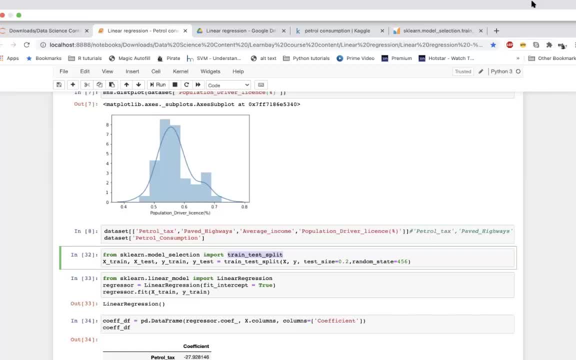 then you're biased in only finding linear relationships. We've not done any kind of exploratory analysis that helps us look for nonlinear relationships, which means that it's good to develop some sort of preliminary insight about something by doing exploratory analysis, But using that knowledge as absolute. 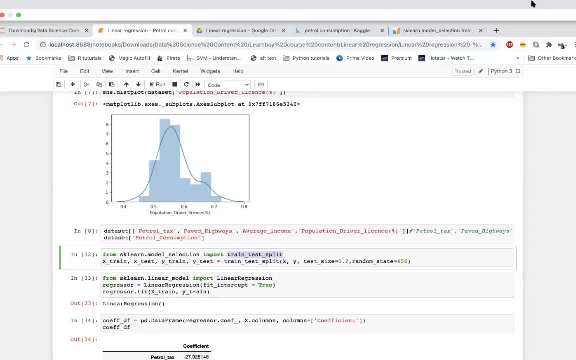 you know facts to help you know, remove certain aspects of the analysis or bring such absolute decisions into play is not a good idea. You know. you should use that knowledge to sort of augment what you learn out of these models, So when you actually build your models,